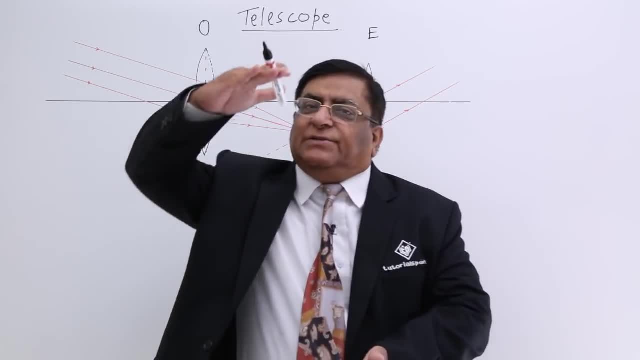 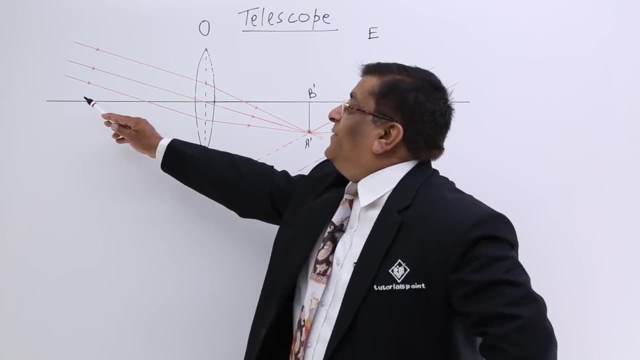 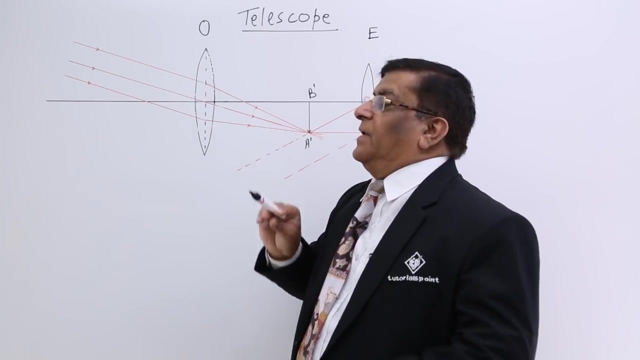 But here what we see, the object is very large and just to calculate the angle, we assume that object is very large. It is so large that the rays are coming at certain angle from there. If this is the object, here is our eyes, the rays will come like this: 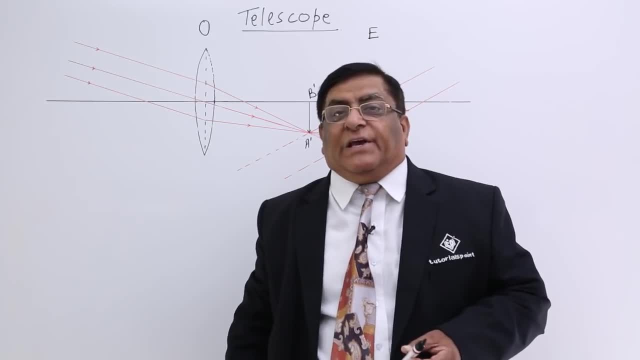 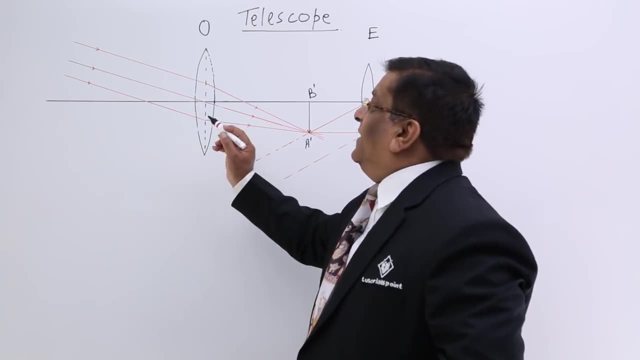 So the rays are making certain angles, So we assume that this is that angle made by the rays coming from the object and they make a certain angle on our eyes and that angle is this. So we give it a name. So we give it a name. 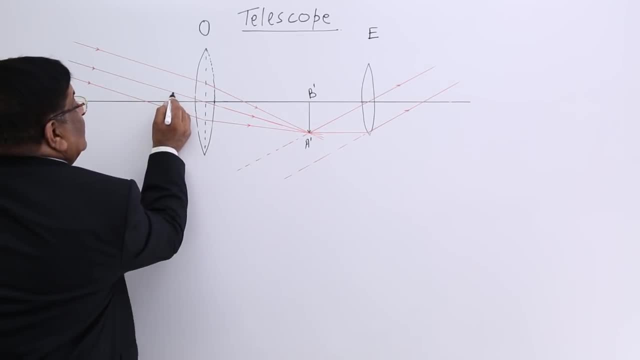 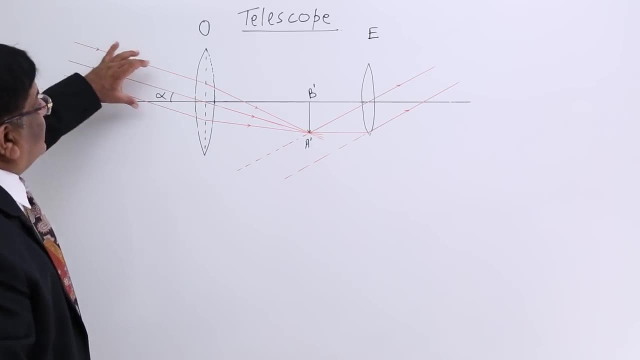 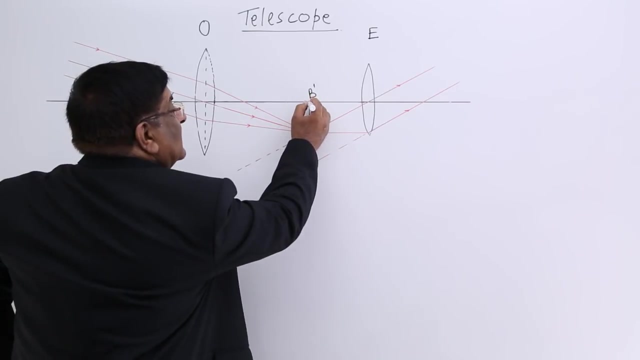 And the name of this angle is alpha, The measurement of this angle is alpha. This is made by object. Now, because they are parallel, they will meet at a point which is on the focal plane. This point is known as focus point, but this plane. if you make a plane here, then that. 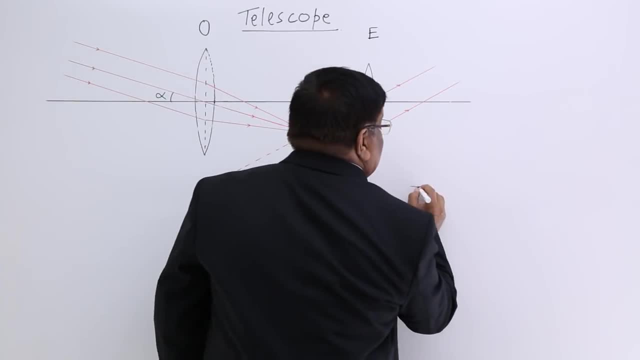 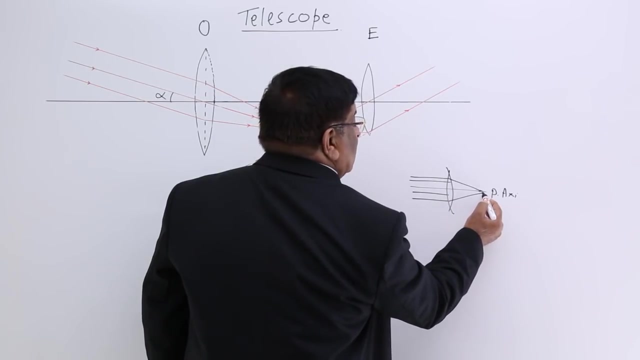 will be known as focal plane If the incoming rays are parallel to the principal axis. This is principal axis of a lens. If the rays are all parallel to principal axis, then after refraction they meet at this point and this point is focus. 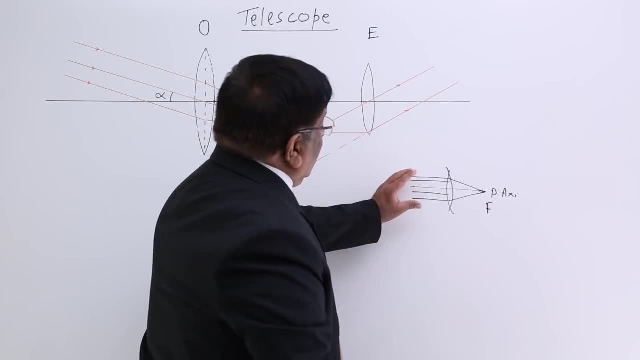 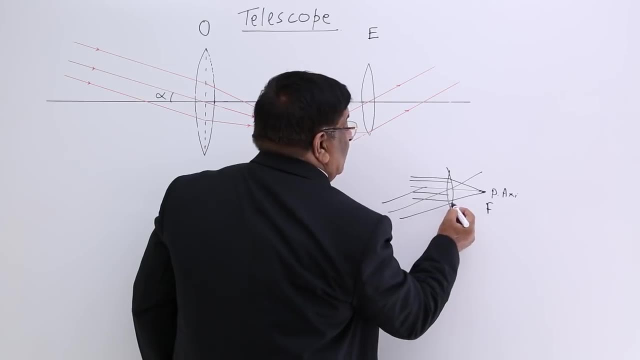 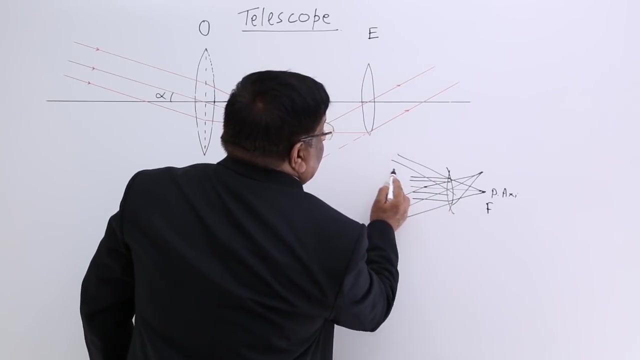 This we have studied Now. if all these rays, I bend it like this: I put a torch and send all the rays which are in this direction, Then these rays will meet at this point. If I bend all the rays this way, Then these rays will meet at this point, here and here. 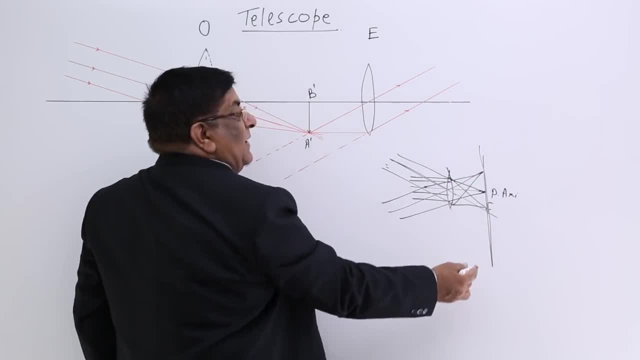 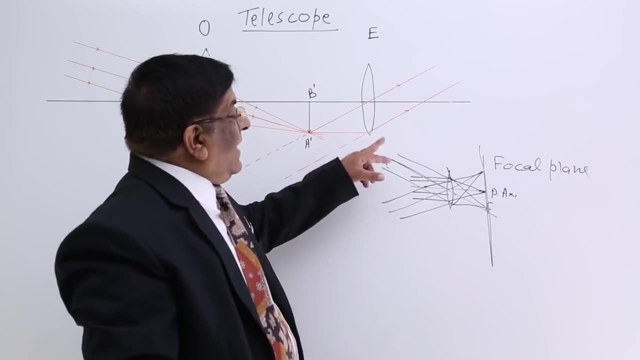 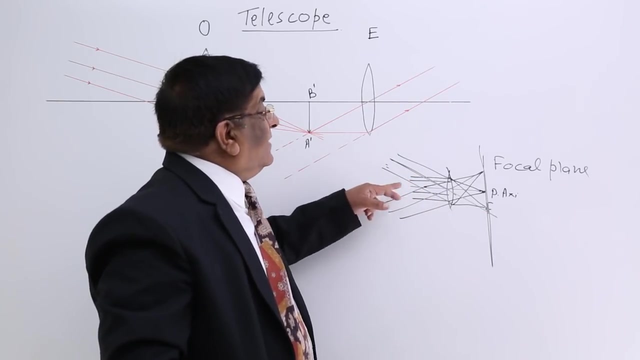 All these points are in one plane and this plane is known as focal plane. So if they are parallel, their point of intersection will be on the focal plane. If they are parallel, and parallel to principal axis, then they will be meeting at a point. 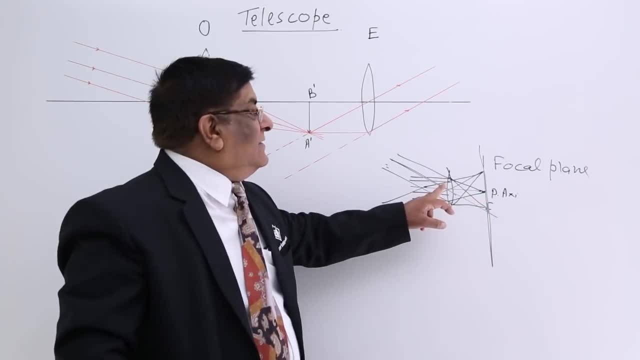 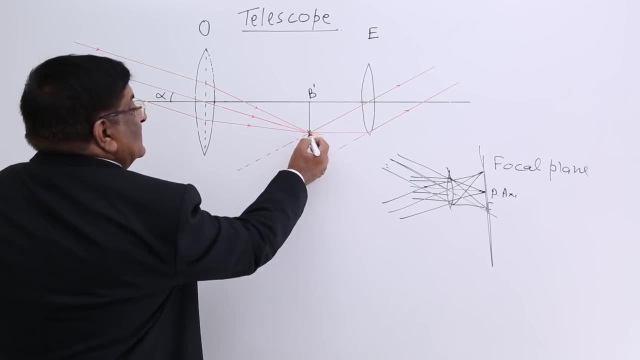 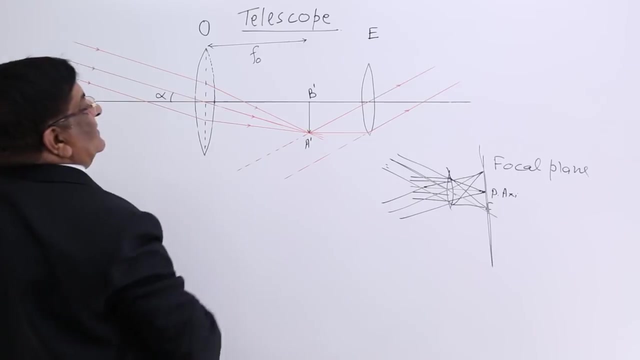 which is on the focal plane. So here they are coming at an angle, So they will meet at a point which is just straight line perpendicular to the focus And this is on the focal plane. So this is focus And focus of objective. 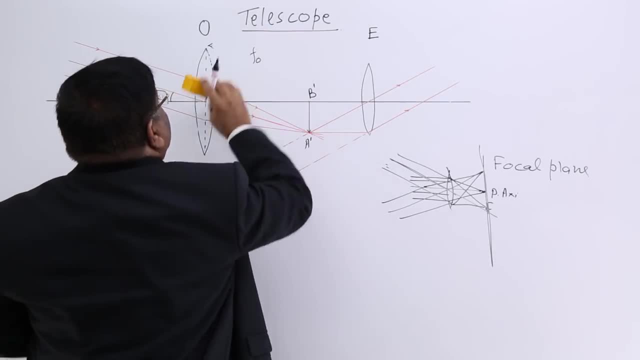 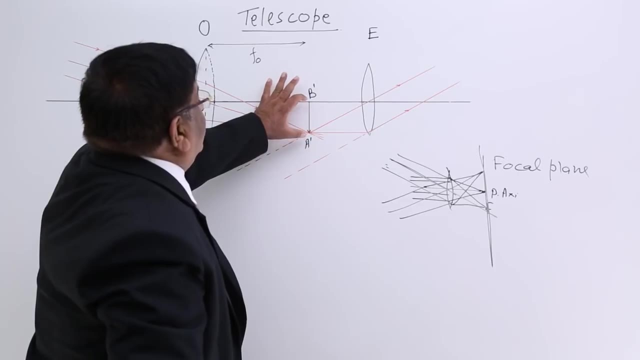 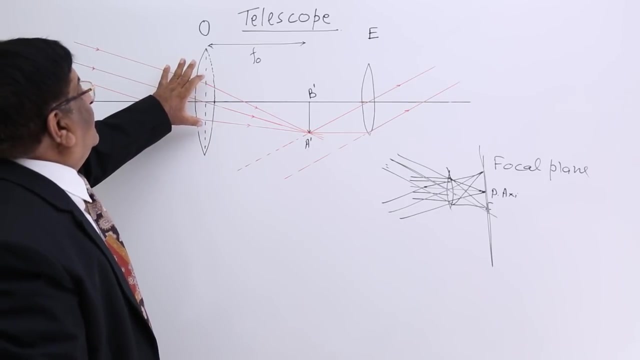 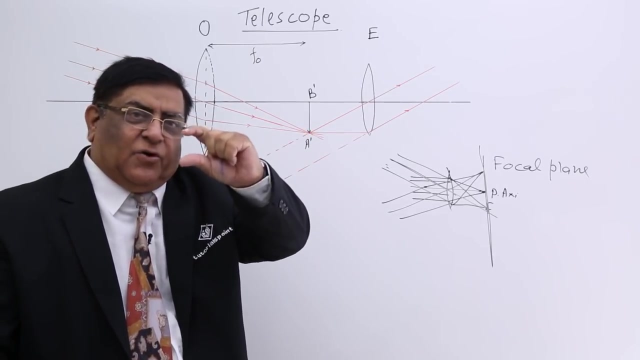 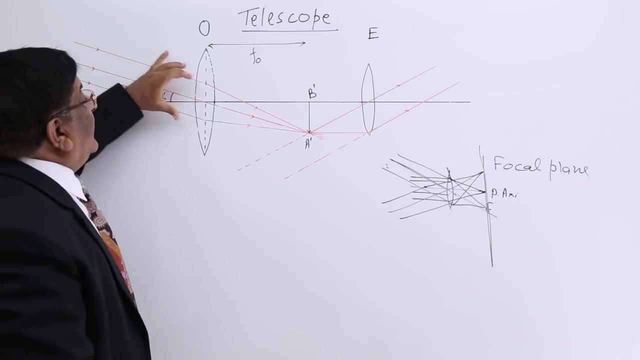 This distance. Now what happens after this? This makes image. So this is the image we are able to make with help of one spherical lens, convex lens. Now this image is quite short and we want to magnify it further. The object of the first objective lens is to create an image. 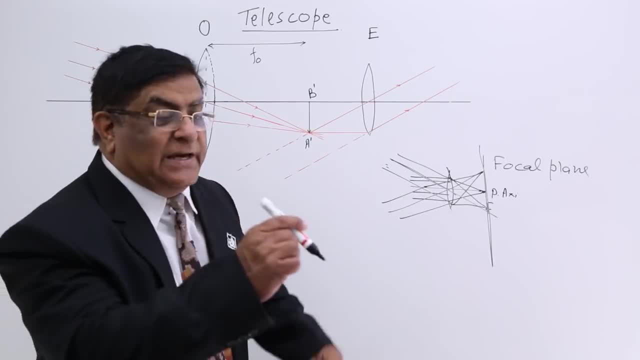 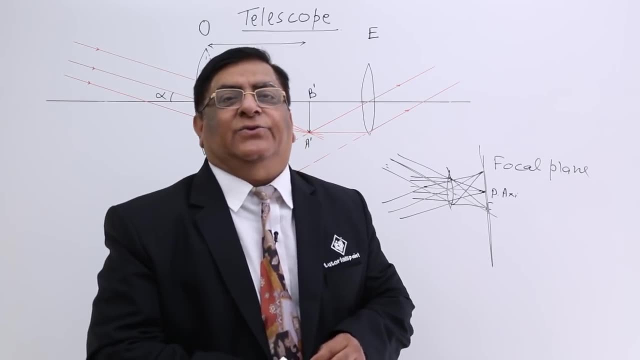 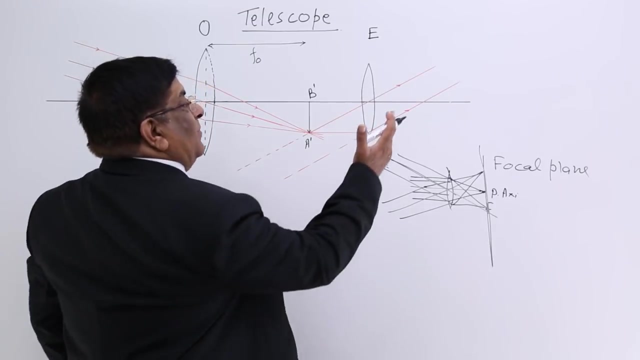 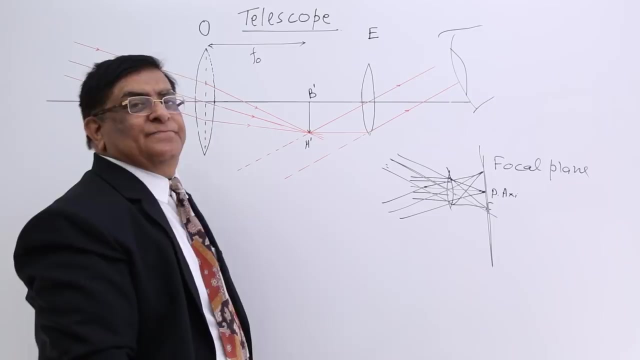 So it will create an image here. Now we want to study that image and to study it I want that this should be large. So for making it large I use a simple microscope and that is a magnifying glass. So this magnifying glass I place here and here I put my eyes and see this object magnified. 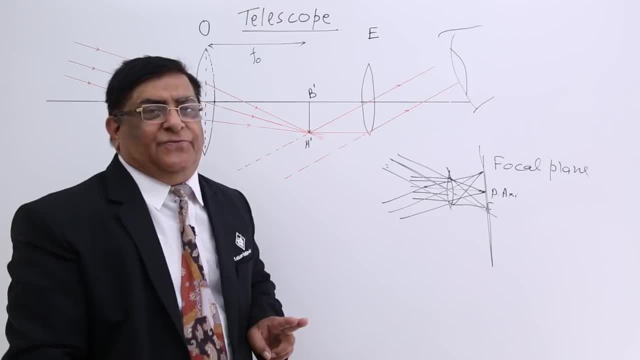 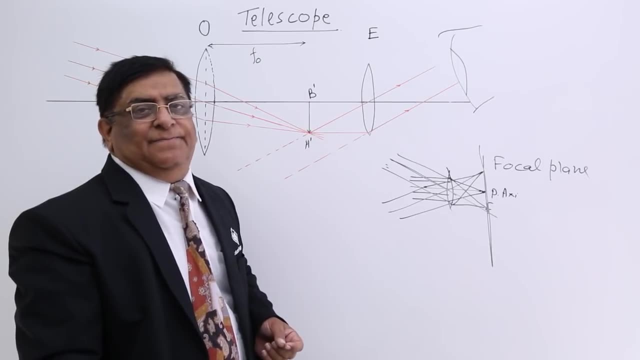 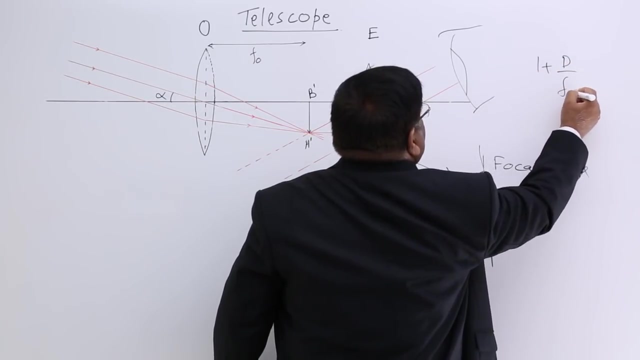 If I want to see this object magnified, there are two type of setting. One is at the distance, One is for distinct vision- We have studied about that- and one is for relaxed eyes. For the distinct vision, its magnification is 1 plus d upon f and for parallel ray setting. 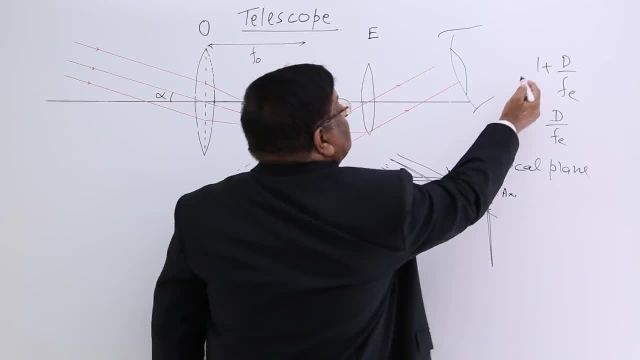 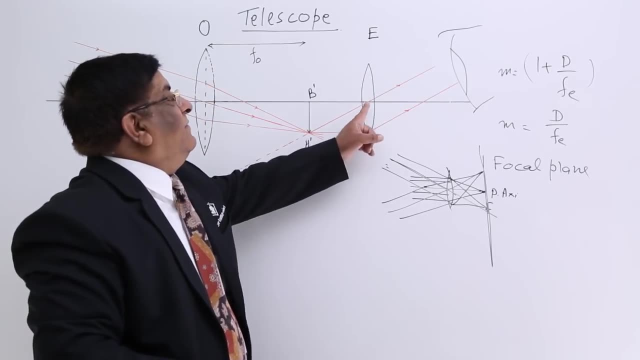 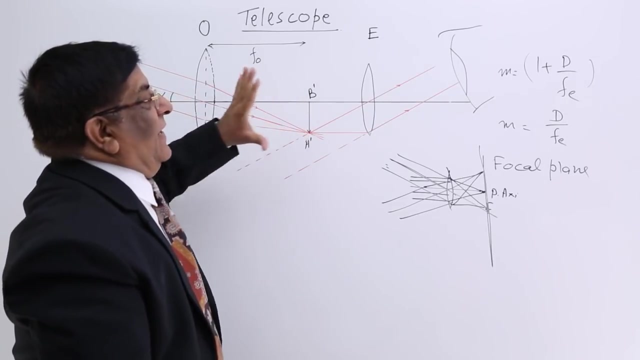 this is d upon f only. So these are measurements of magnification of this simple microscope. Here we are calling it eyepiece because it is close to the eye. So this is magnified and we see the magnified picture of this image. and this is the image. 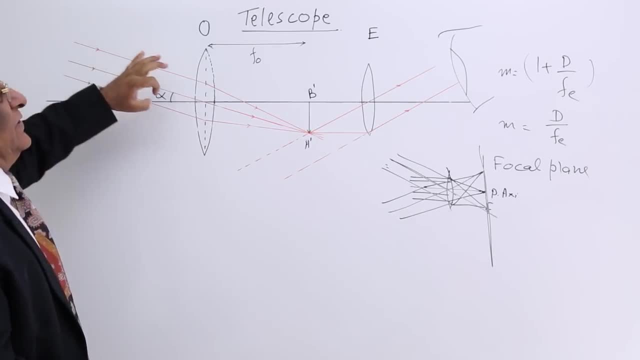 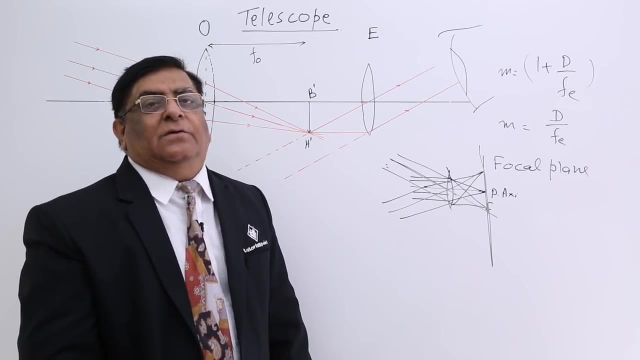 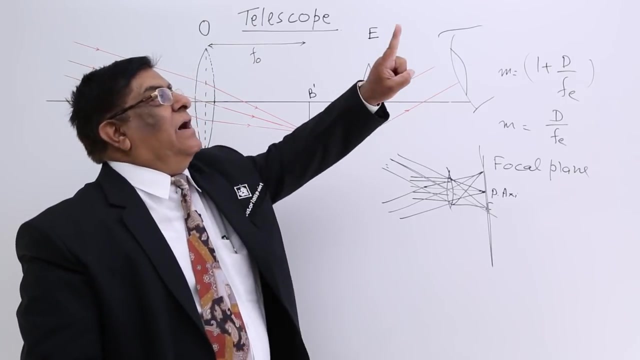 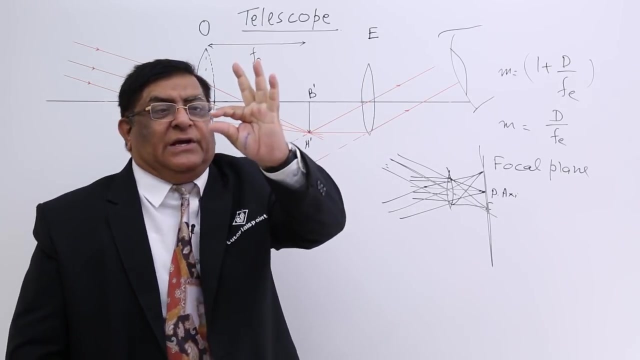 of certain planet or star which is on this side. So this is the action in telescope. You can ask whether really the image has been magnified. Yes, Because when you see the star without any instrument, You see it just like a point, and when you see it in the telescope it is much larger. 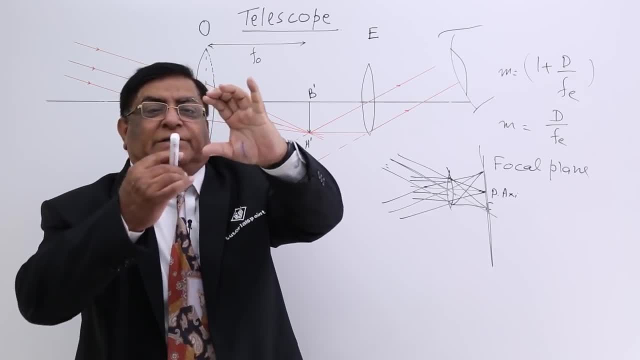 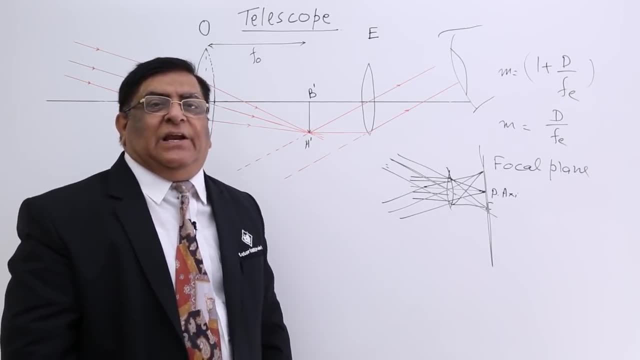 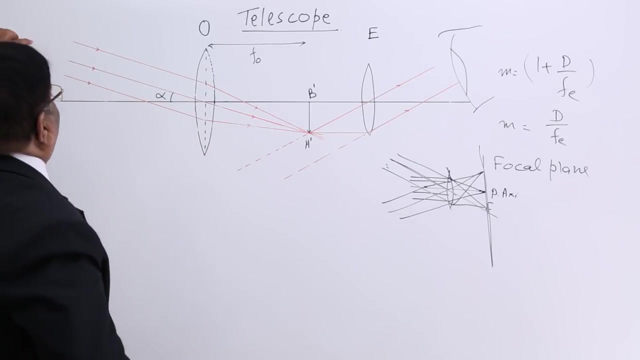 Even if it has come become like this, compared to a point, this is very large. This is magnification done by telescope. Is there any physical proof that this will really become large? Answer is yes. The angle subtended by the object is alpha. 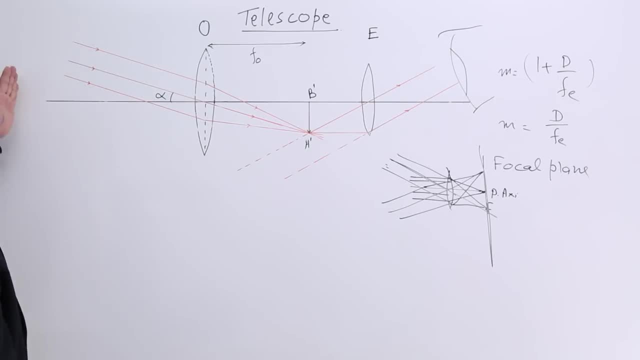 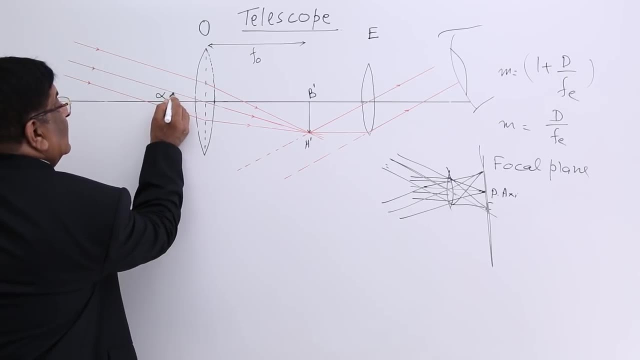 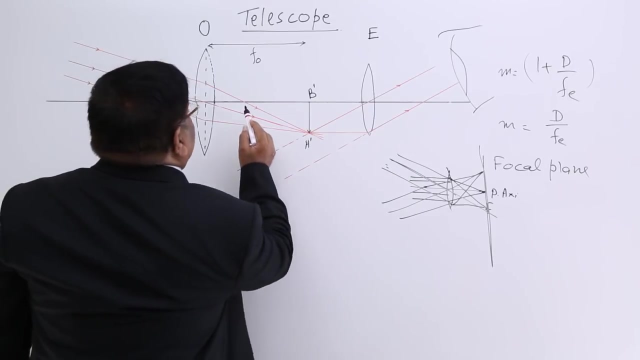 Object becomes larger, Object is the infinity is very large. These are the rays coming from the top end, from bottom end. So this is alpha: is the angle made by the object. we assume Then this ray which is coming from the bottom of that object. 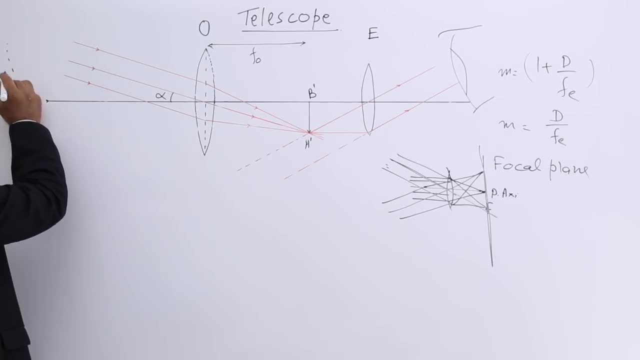 This is from top of that object, and that object in the sky is somewhere like this, Yes, Far away from the top, from the bottom. This is direction from the bottom and this is alpha. This is angle made at the eye. You can say: eyes are here, how? this is the angle. 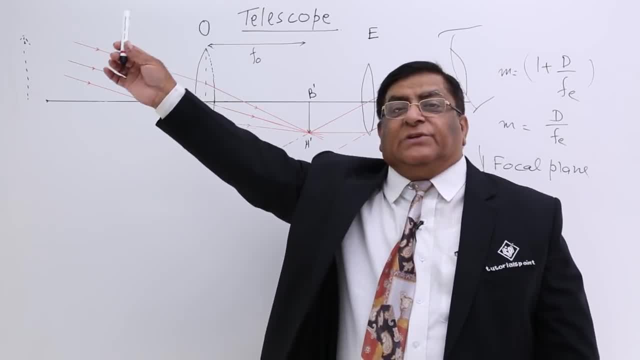 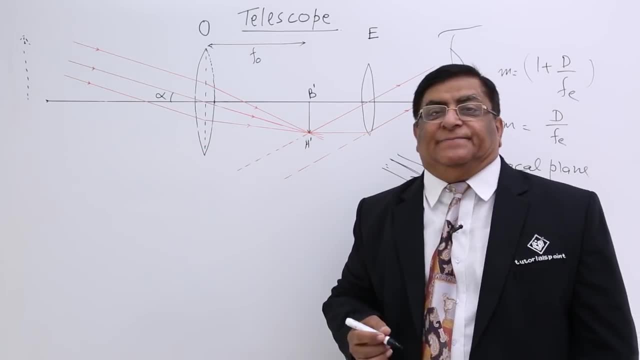 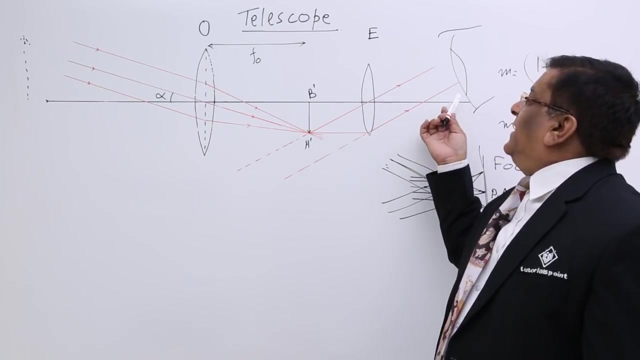 The answer is: these rays are coming from thousands of miles, millions of miles away. For them, this distance or this distance does not matter. So Whether they make angle alpha here, They will make the same angle alpha here, They will make the same angle alpha on our eyes. 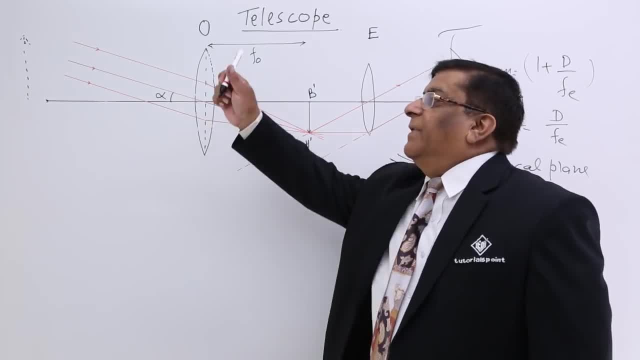 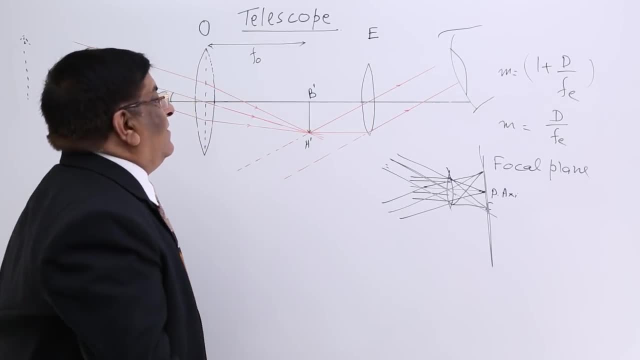 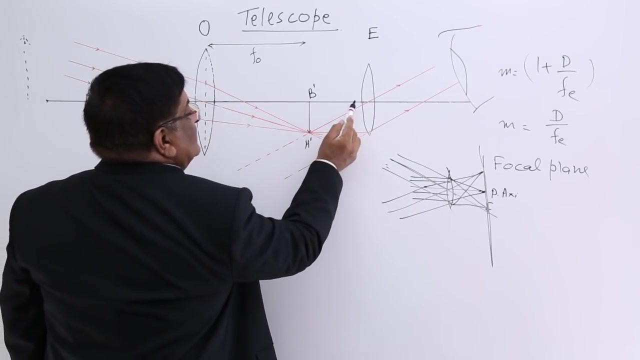 So this can be treated as angle alpha made by the object on our instrument, on our eyes. Okay, Now what is the angle made by the same image on our eyes? Answer: this ray is common, straight coming from the bottom of the object And 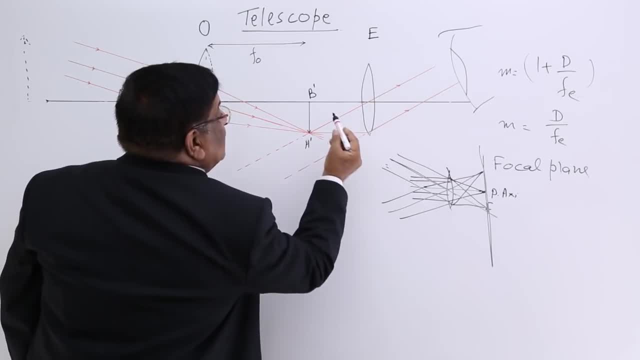 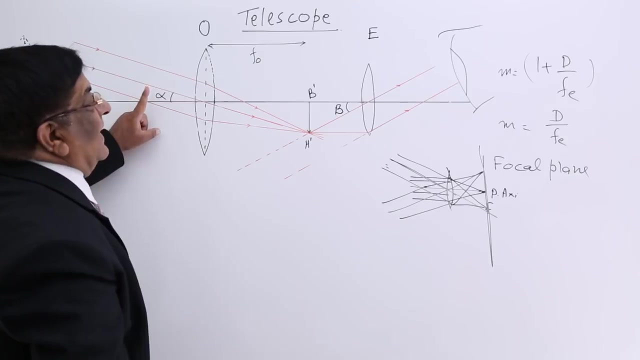 This is the ray which is going to my eyes, Then this is the angle subtended by image on the eyes, and let us call it beta. Okay, Now, if beta is larger than alpha, Then this is magnification, and we can see beta is larger than alpha. 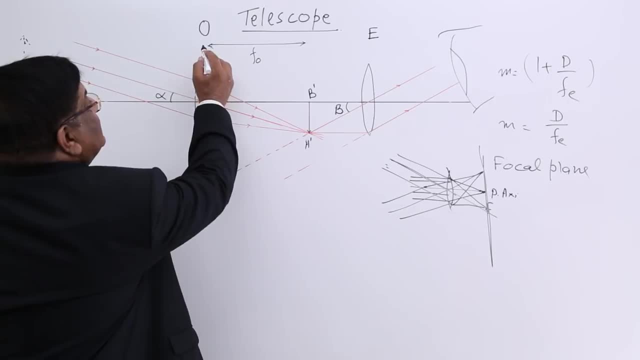 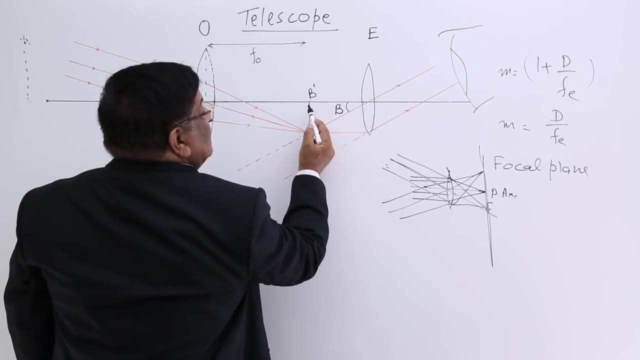 How beta is larger than alpha, Because this f ohm. And how much is this distance? This is also focal length of this. That is why the rays going from here has become better, So this has to be at the focus of this. 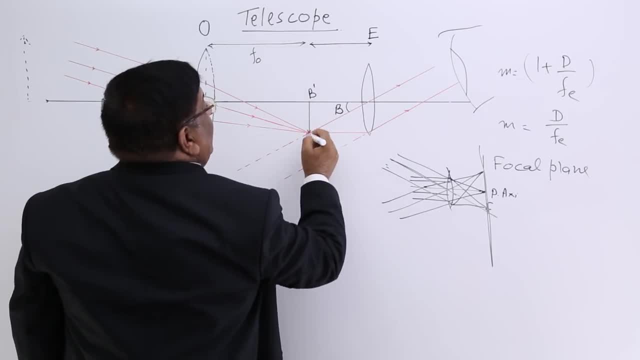 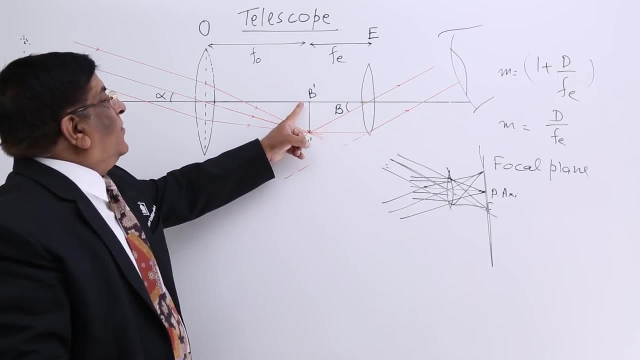 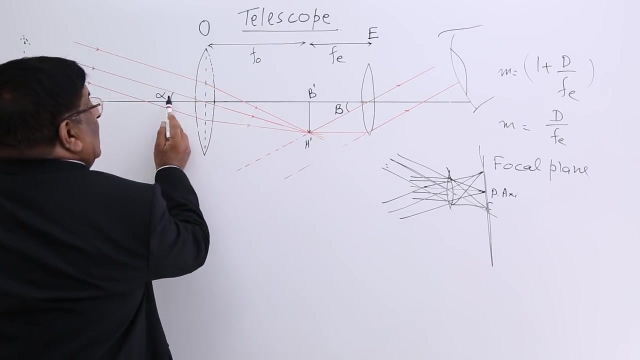 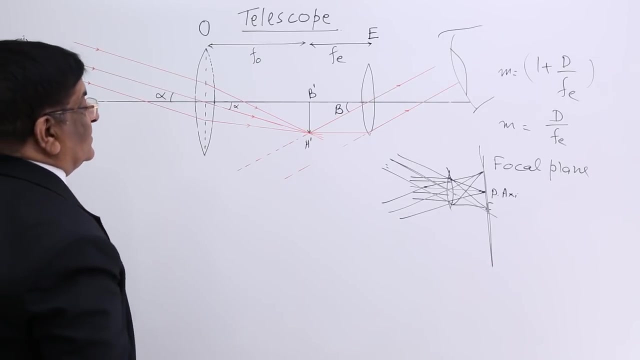 So this is focal length of eyepiece. The focal length of eyepiece, we take small. The focal length of object, we take large. So Beta, Beta upon alpha. This is alpha, So this is also alpha. So what is magnification in this case? 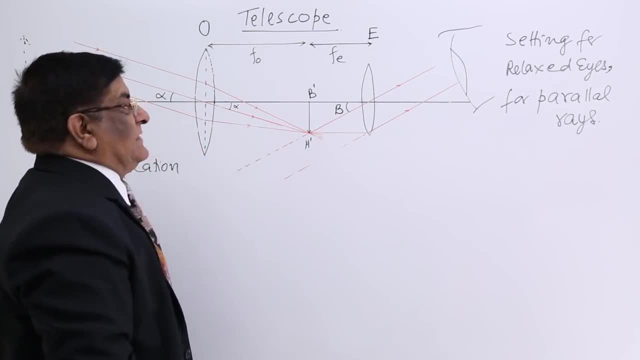 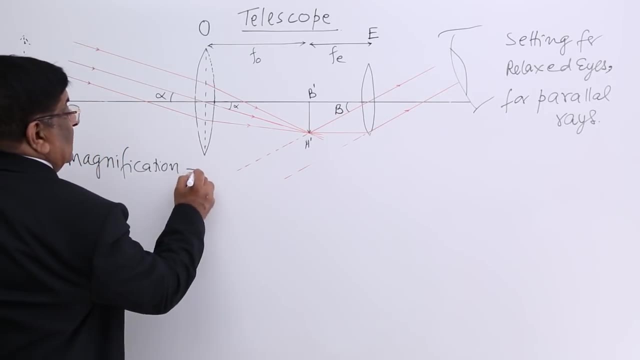 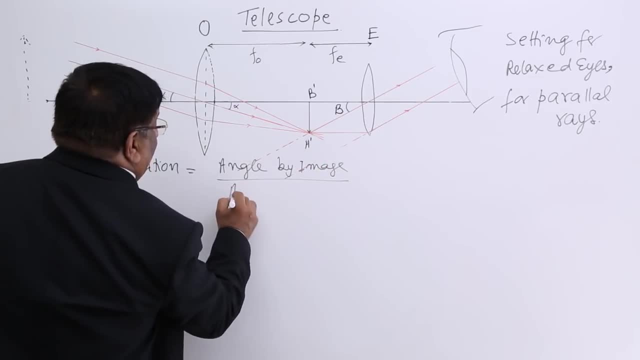 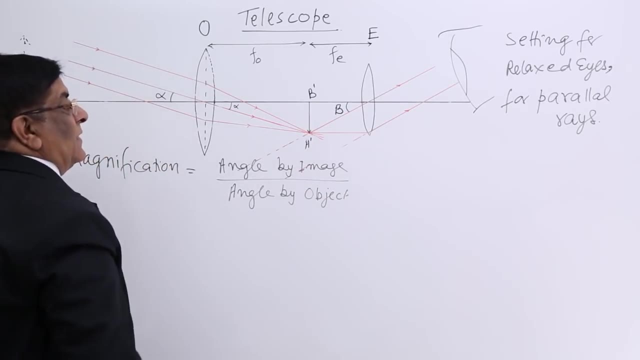 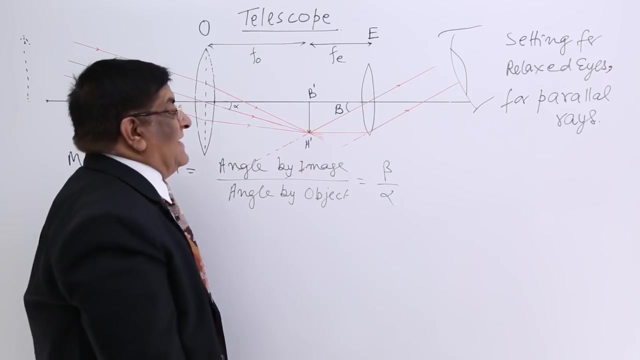 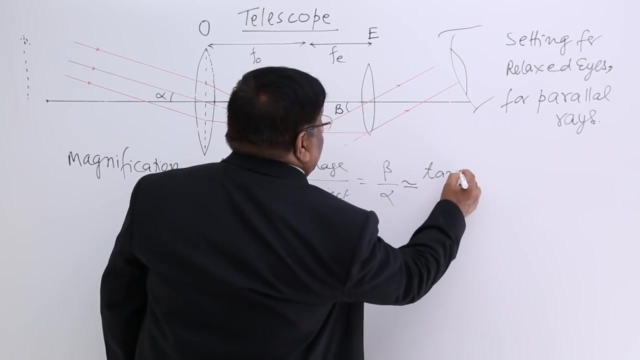 This is the angle On the eyes divided by the angle subtended by object on the eyes. Here it is beta upon alpha, And for small angles we can take them as tangent Tangent beta upon tangent alpha, Tangent beta upon tangent alpha. 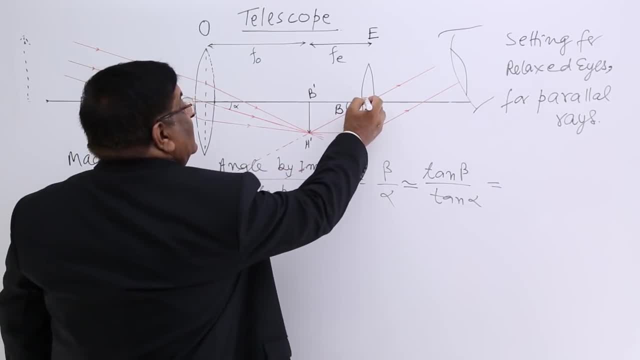 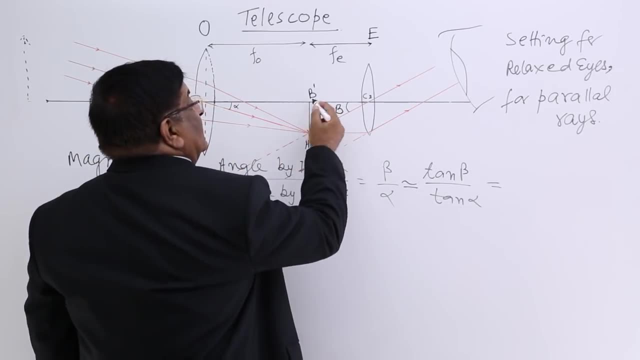 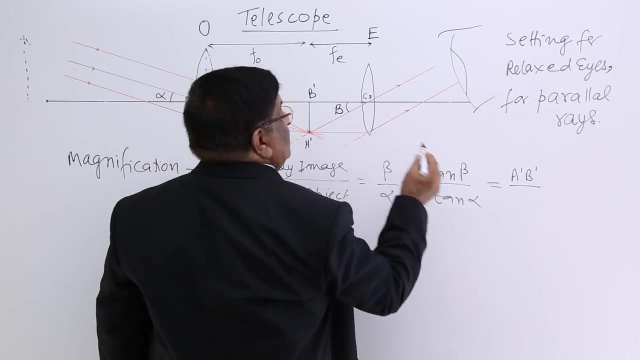 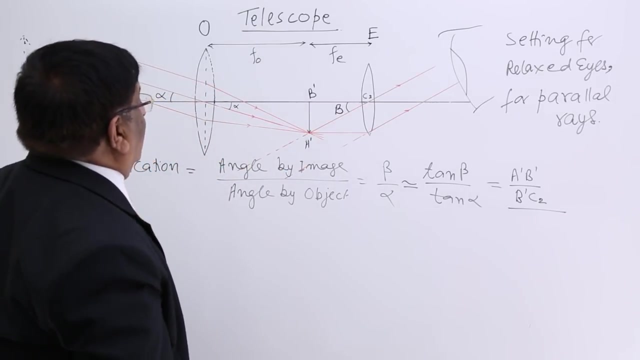 Tangent beta upon tangent alpha. Now tangent beta Decreases, Decreases, Degrees. take it as: c 2 b dash upon a dash, b dash. sorry. a dash b dash upon b dash c 2. a dash, b dash upon base b dash c 2. this is tangent beta. this is to be divided by tangent alpha. this: 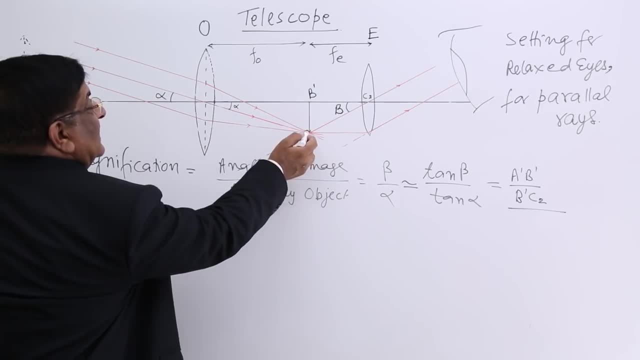 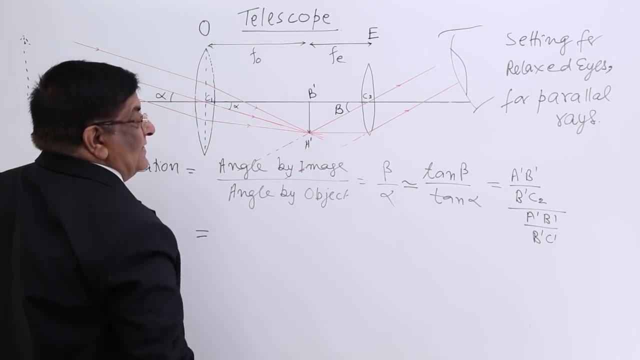 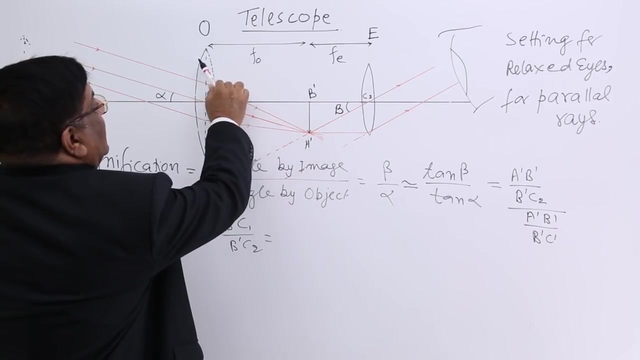 is alpha. opposite angle: this is alpha and it is tangent. is a dash, b dash upon b dash c 1, cancellation of a dash, b dash, and what we get is b dash c 1 upon b dash c 2. now b dash c 1, b dash c 1. this is focal length of objective and the sign is positive on this. 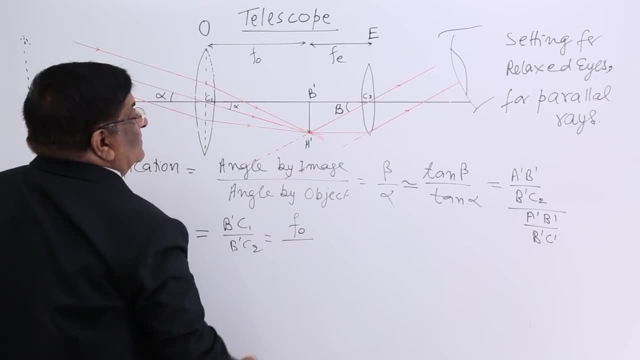 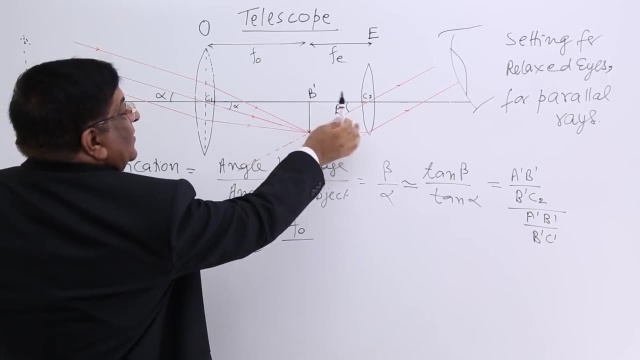 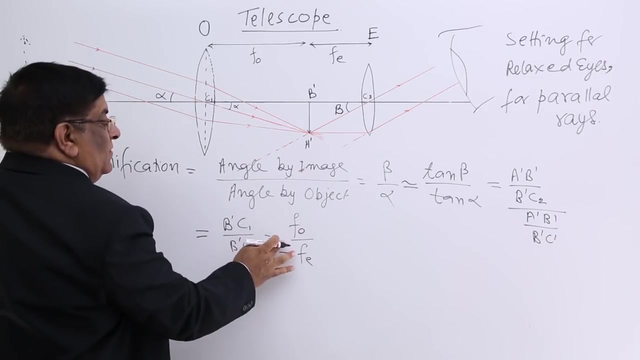 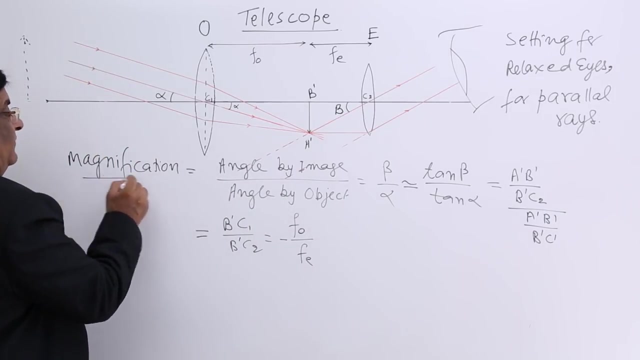 side. So while putting the value, this is fo b dash c 2. b dash c 2 is focal length of ips, but it is on the left side, on the opposite side of incoming rays, so this is negative fe. so we got the formula here: this is minus fo upon fe. what is that magnification? 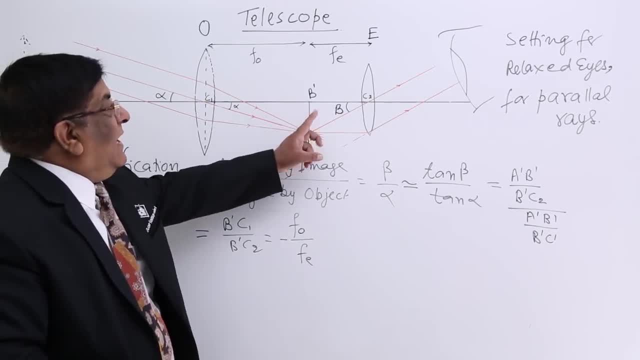 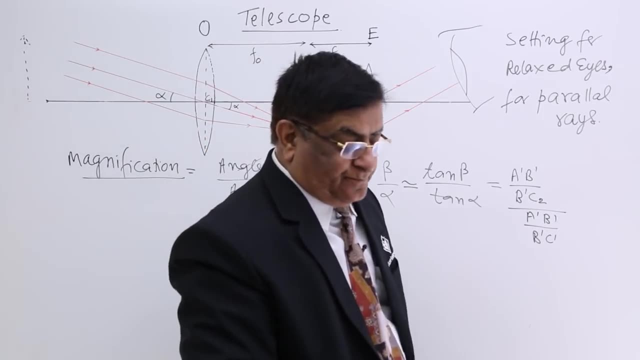 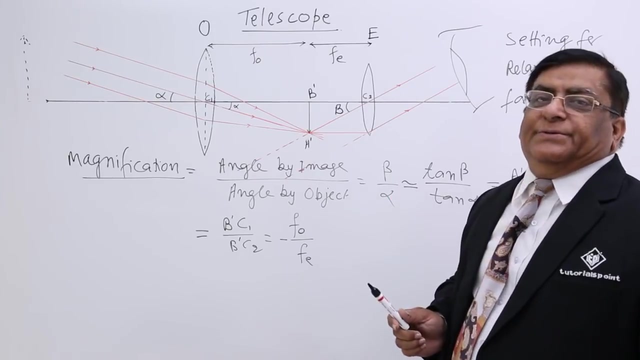 Now, if we have taken fo as large one and fe as small one, Definitely there is a magnification of more than one. So this is how we magnify with help of a telescope. Now, in this telescope there are few features. we understand one thing: that fo should be. 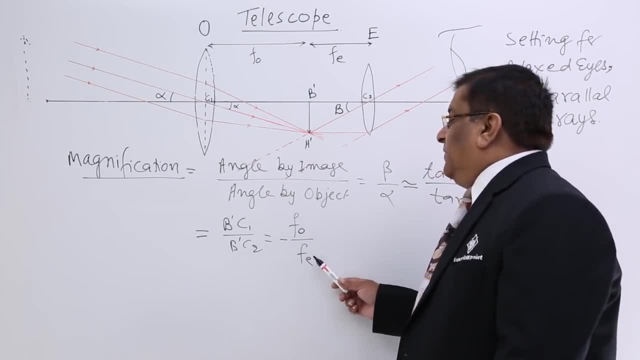 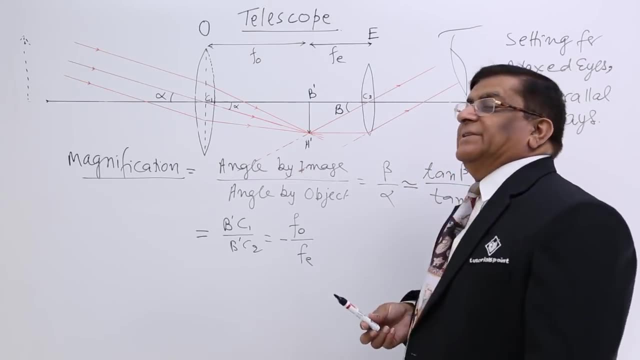 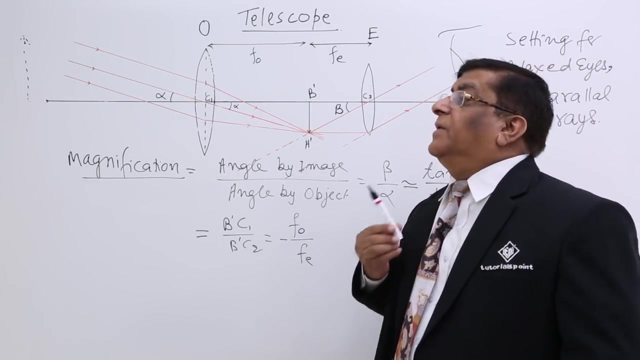 larger than fe. fe should be as small as possible. fo should be as large as possible. If we take fo very, very, very large, Then Is there any problem? answer is yes. we have to use a very long pipe and there is a limit of the long pipe. you can use 1 meter pipe, 2 meter pipe, not more than that. 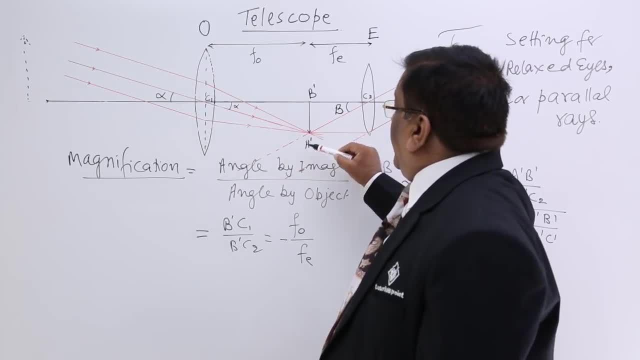 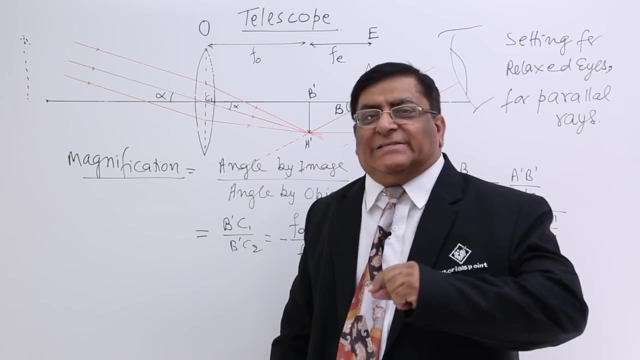 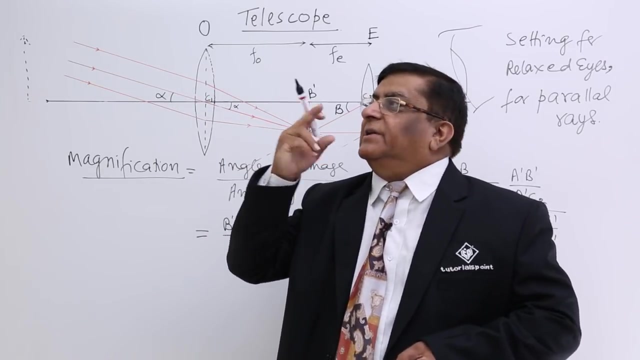 Other thing is that these rays, when these are magnified here, say we magnify it 20 times, then the brightness will decrease by 20 times because the same rays. we are not increasing the number of rays Initially. when we see the star it is giving certain brightness because all the 100 rays 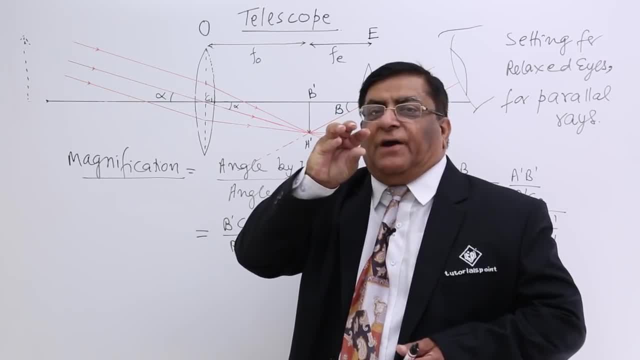 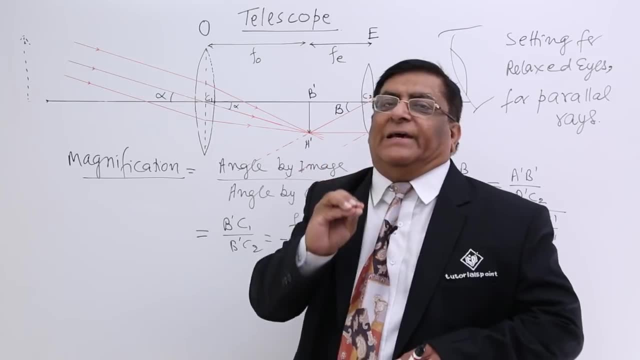 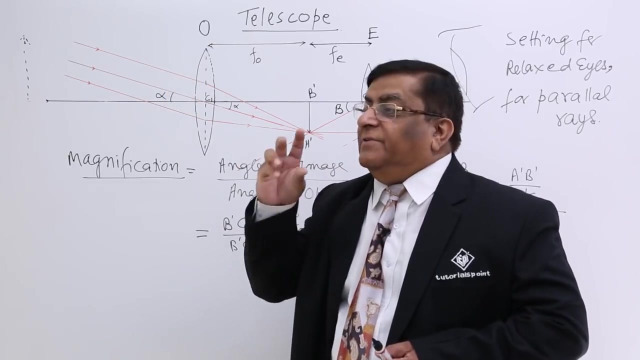 are in this area. Now, when we magnify it, the image becomes this large, but the rays remain 100. So their density will become less and they will appear darker. So when we see the star it is bright, but when we see it in the telescope it becomes a bit. 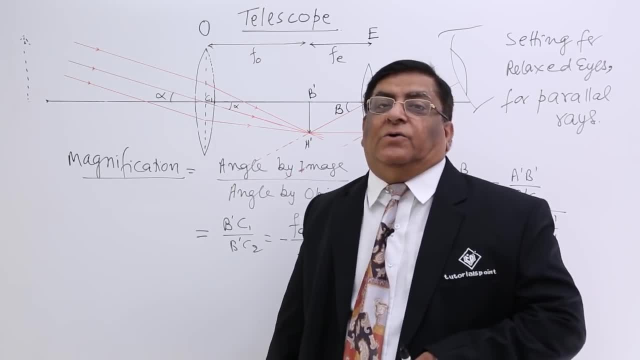 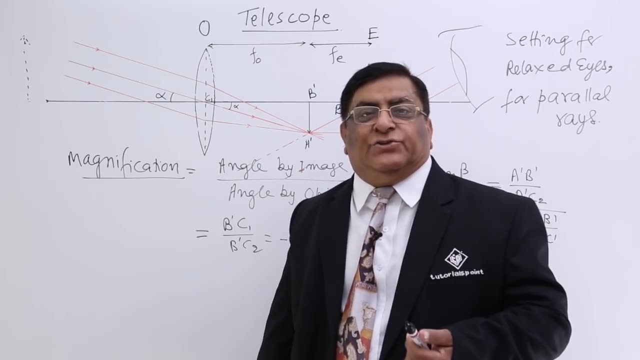 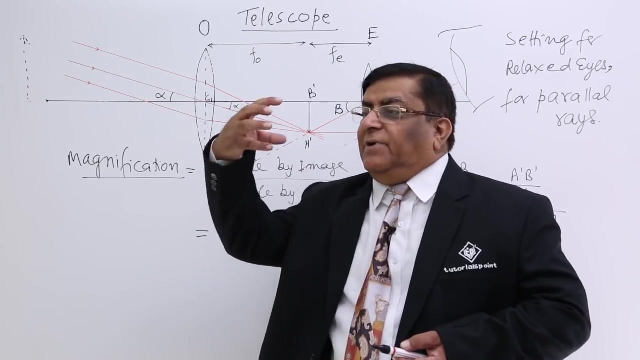 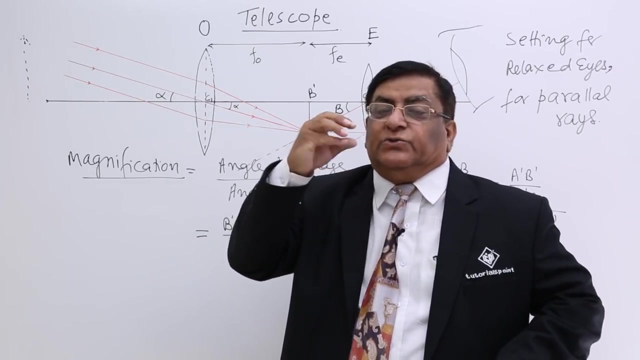 darker because we see larger. Ok, Now to make this effect less. we want to see brighter and brighter image. What should we do? Answer is: we should collect more and more rays So that, even in such a ray, the rays which are coming are 100. we want to make it 1000. 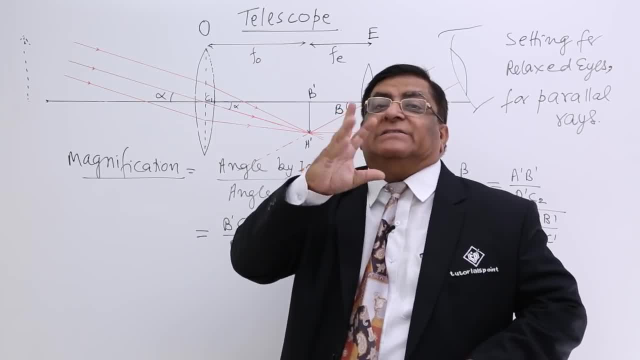 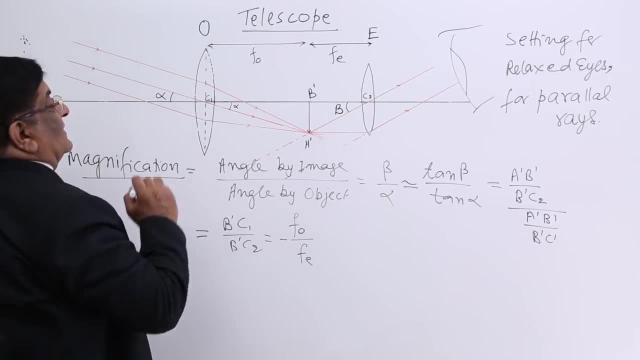 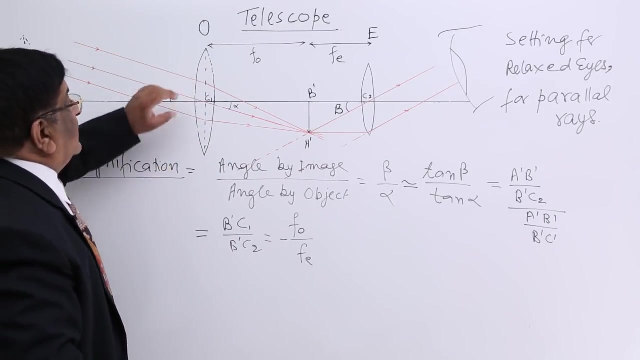 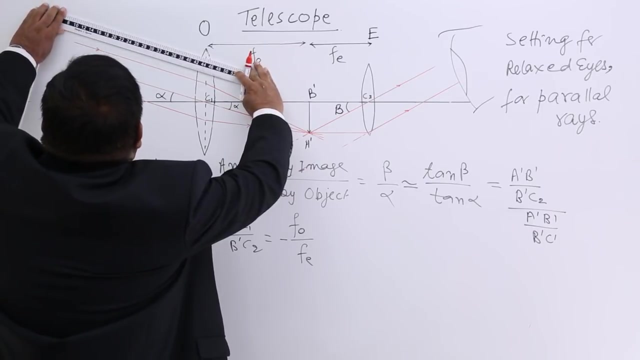 So that when we magnify it, the intensity does not fall. So what do we do? This area we increase. Suppose we have this much of lens and it is collecting 1,, 2, 3 rays. Now we have this much of lens and this lens is collecting a large number of rays. 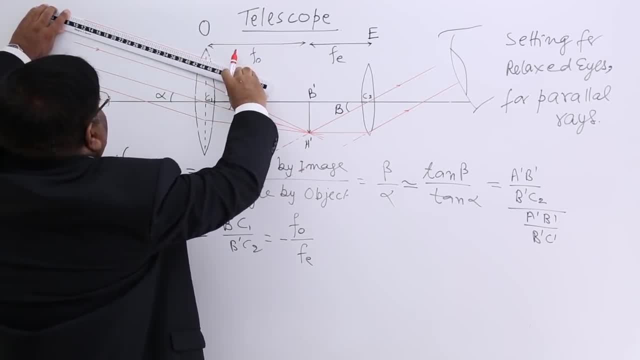 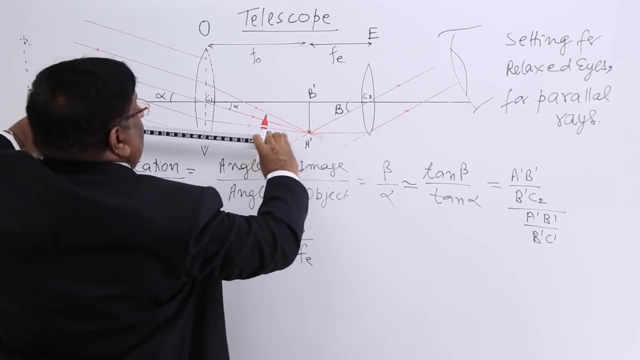 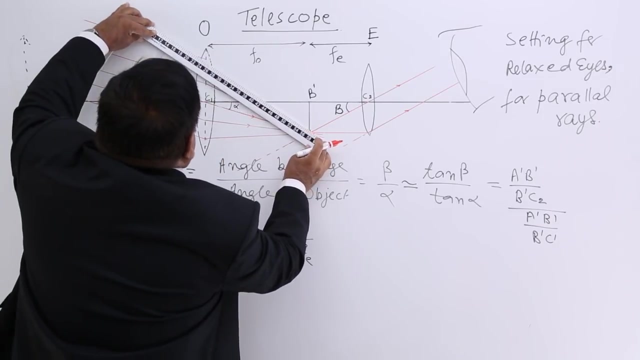 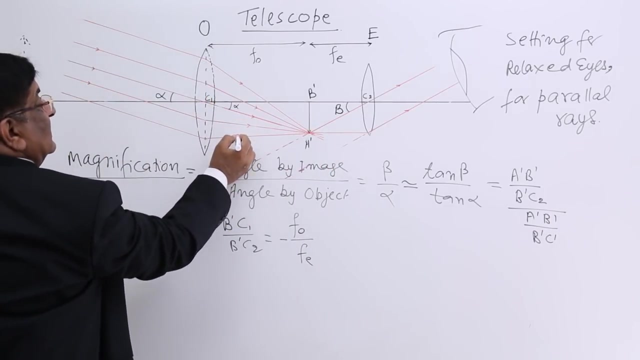 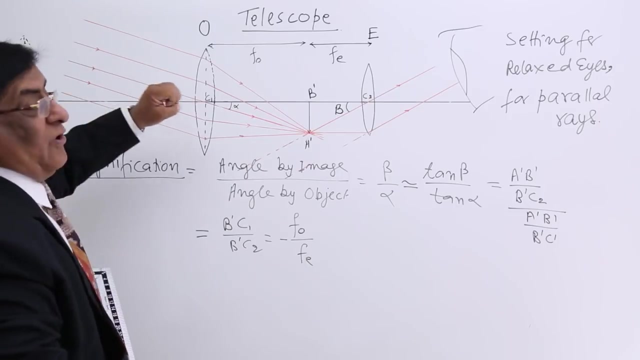 Suppose it can now collect this much. So here, Ok, Ok, Ok, What we find? That there is a collection which is double than the previous collection, So its brightness has increased twice. Now, if I increase this area 100 times, then the total rays will also increase 100 times. 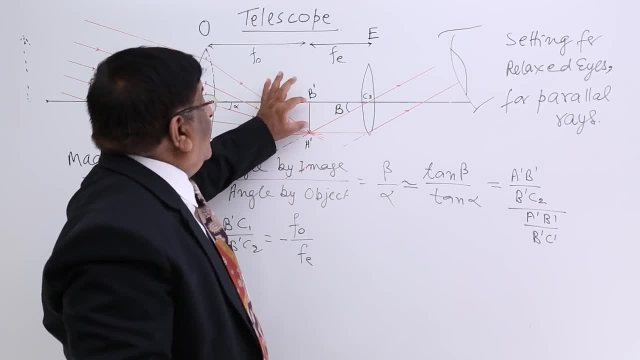 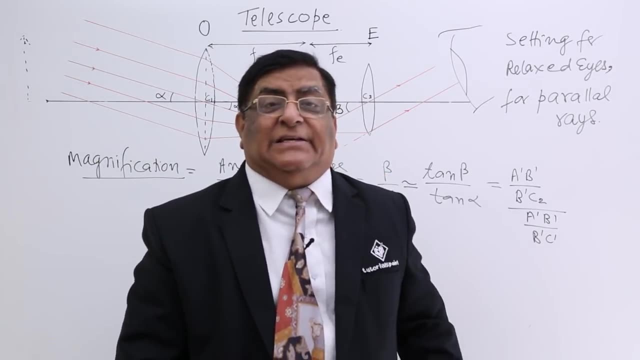 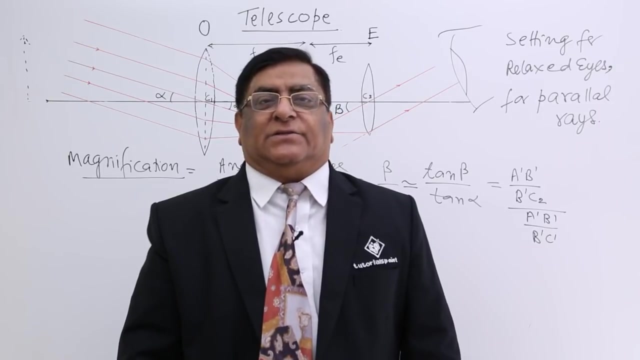 Then this image will be very, very bright and even if I see it larger, magnify, it will be magnified, The intensity will not decrease much and I will be able to see it. So with this we understand one characteristic of telescope, that objective of the telescope. 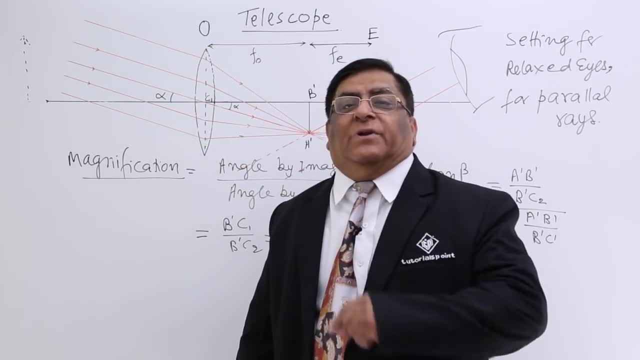 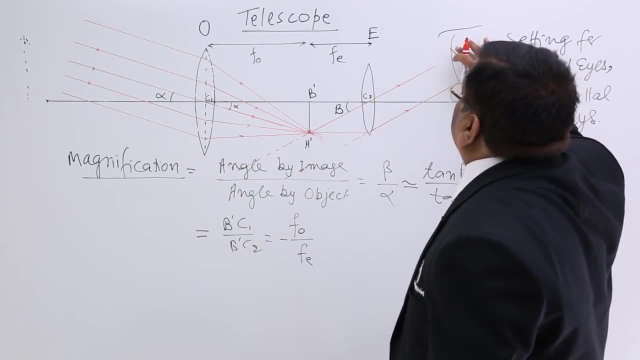 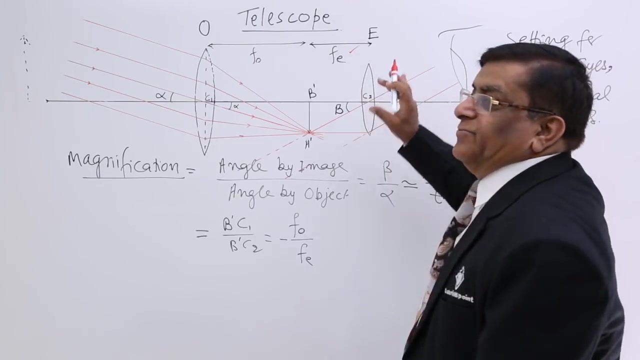 should have as large aperture as possible. So that is why this lens is large aperture, For this it should only accommodate our eyes and its focal length should be small. For small focal length we cannot make very small, we cannot make very large apertures. 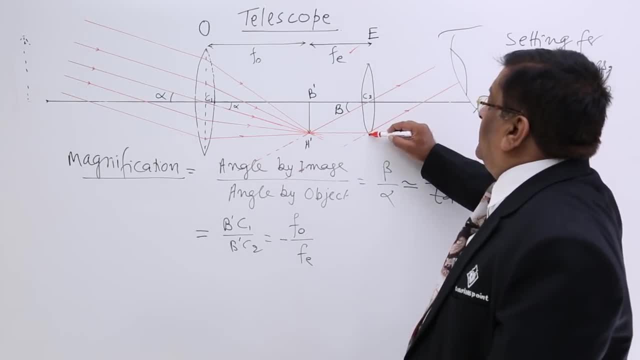 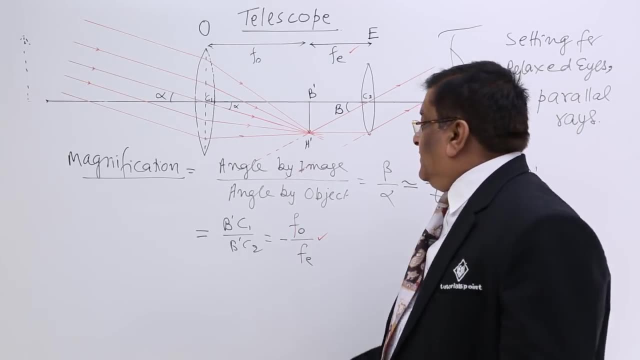 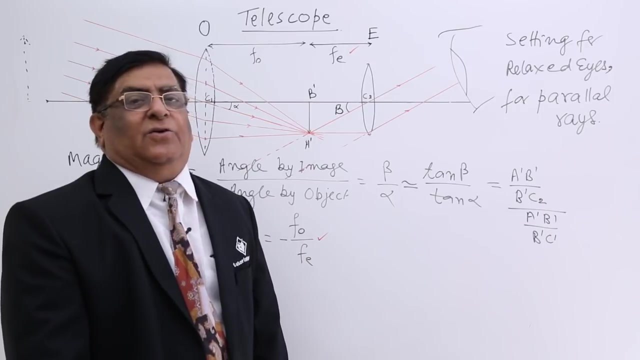 We have to make the aperture small. So this is a smaller lens, this is a larger lens and this is magnification. Now, in this magnification, we understand this. Can you compare it with magnification of microscope? Microscope is also made by the combination of two convex lenses, but in case of microscope, 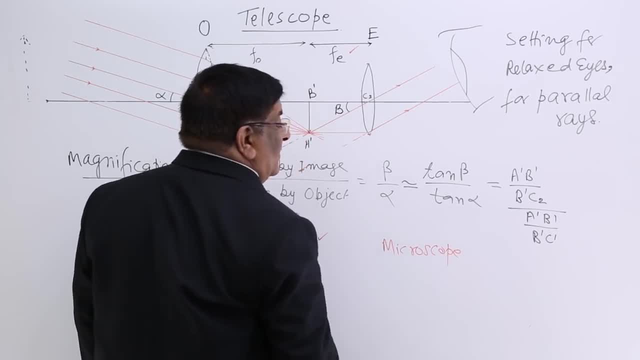 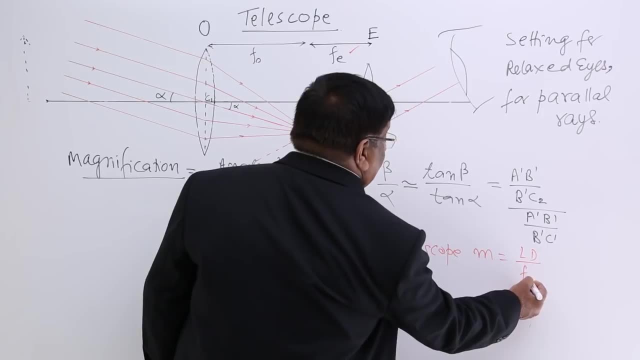 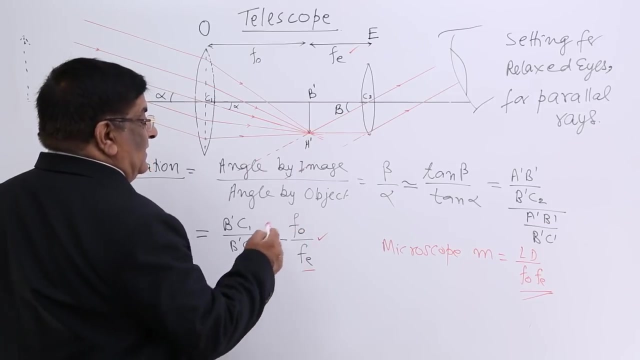 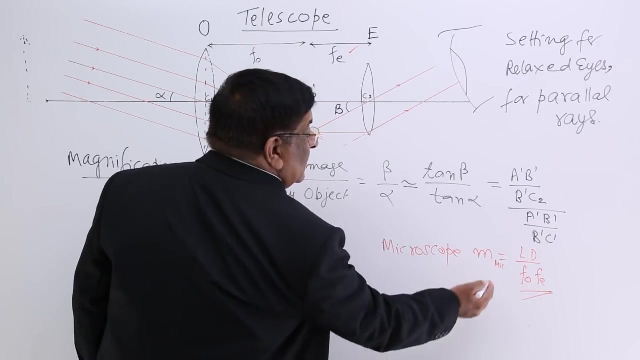 that is compound microscope. we have seen that magnification is something upon Fo into Fe. Both of these are in denominators. Here only this is in denominator, this is in numerator. So magnification of microscope Fo should be as small as possible In denominator. 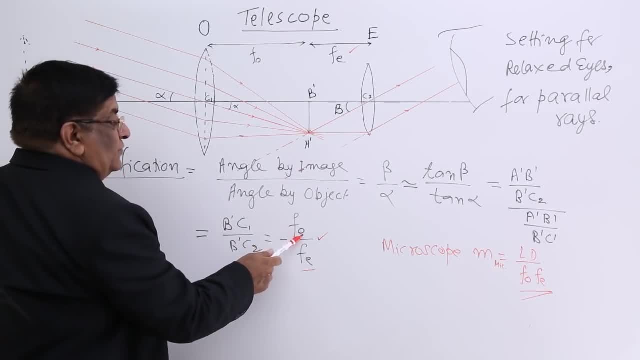 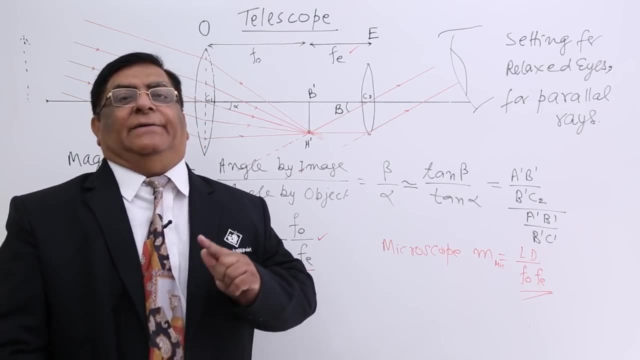 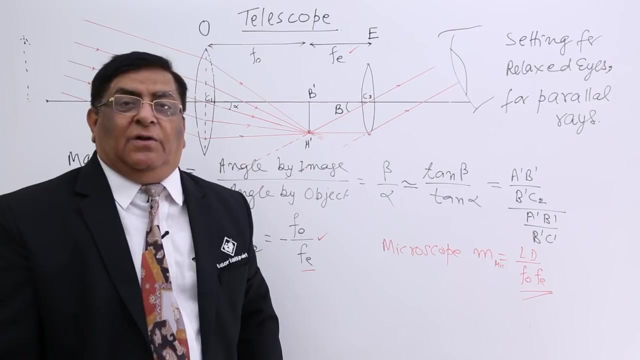 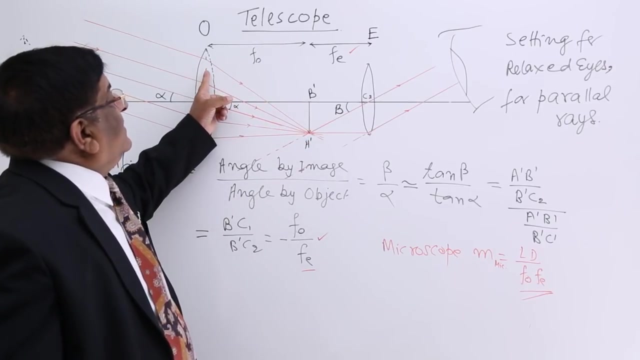 Telescope magnification, Fo should be as large as possible. This is the basic difference in telescope and microscope. So if somebody ask you why telescopes are long and microscopes are small, The answer is: in telescope we have to accommodate inside the focal length of objective lens and 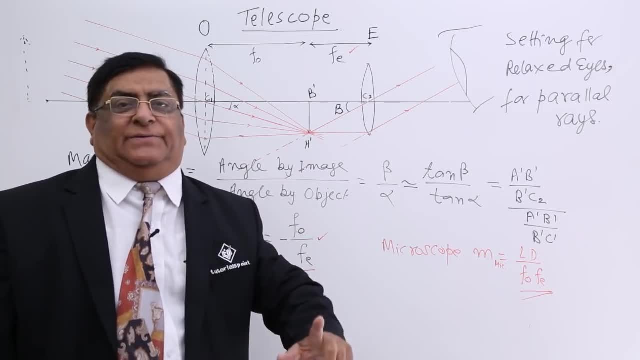 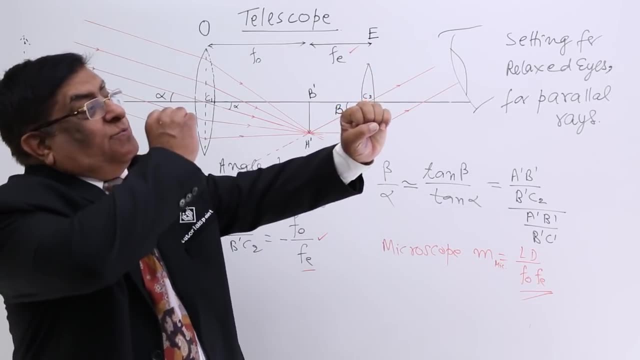 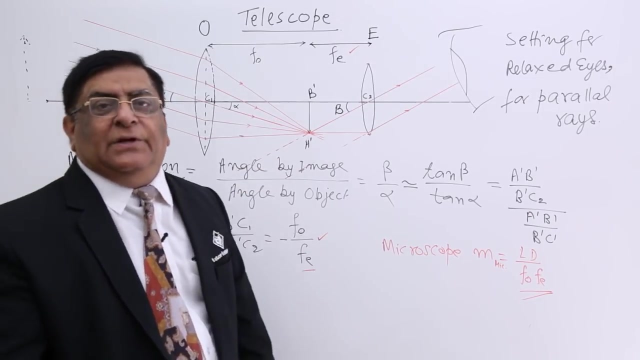 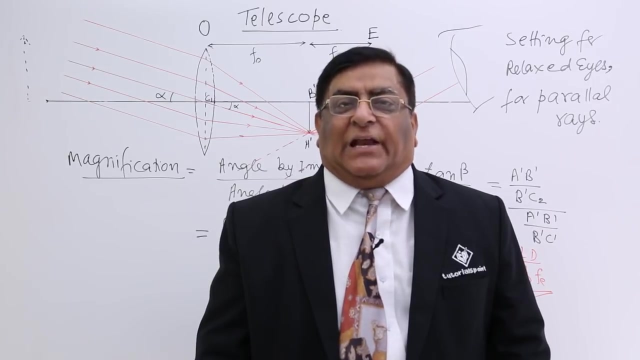 the focal length of objective lens has to be kept larger. That is why we have to make the pipe very long and that is why the telescopes are very long pipe machines. So this is about the telescope. Now in the next lecture we will see what are the probable defects in this telescope and 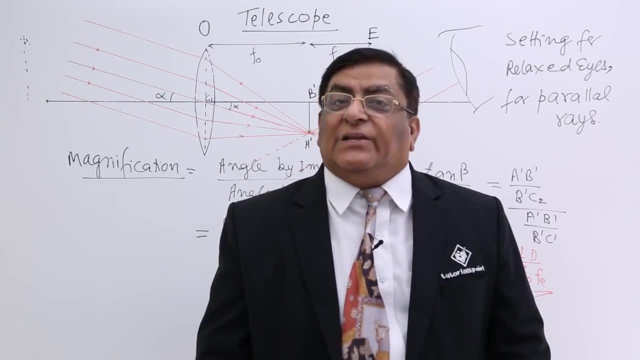 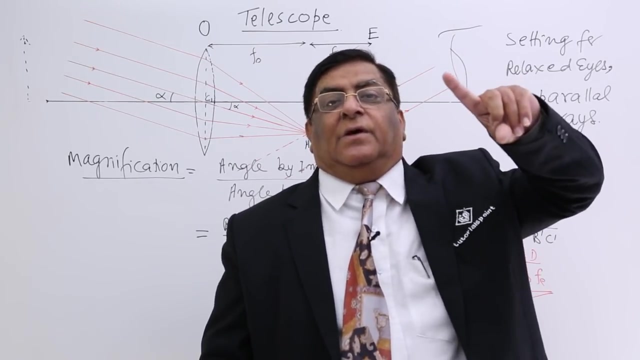 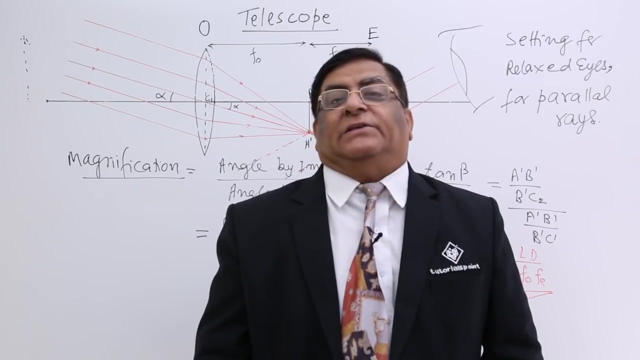 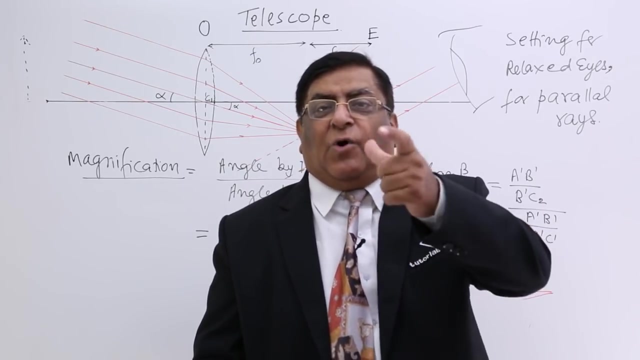 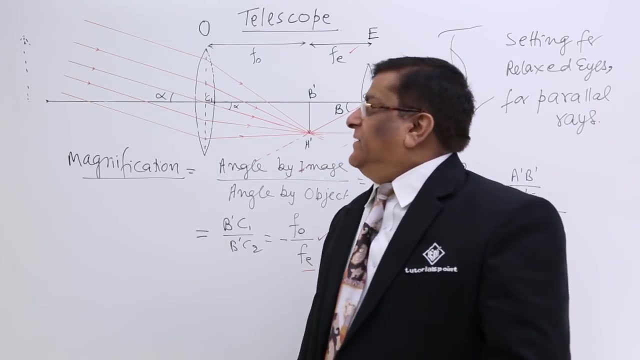 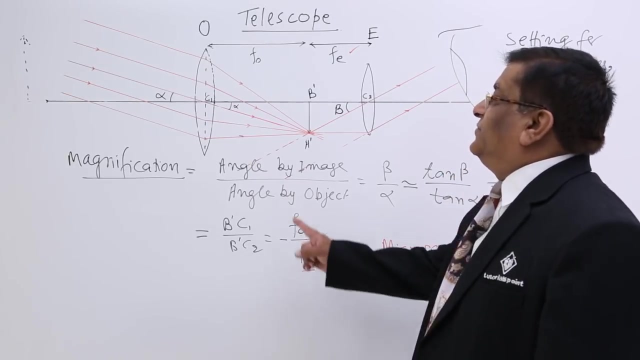 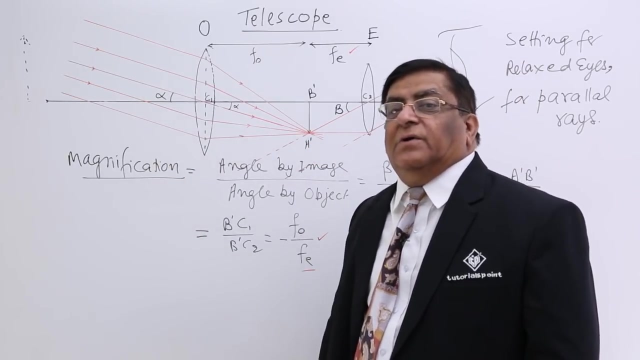 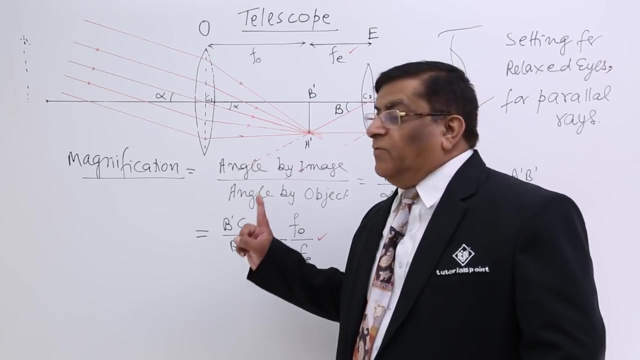 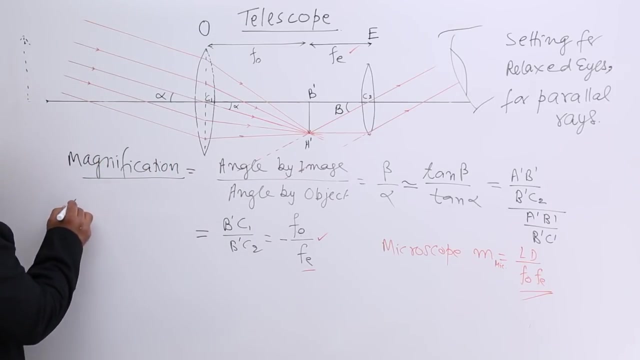 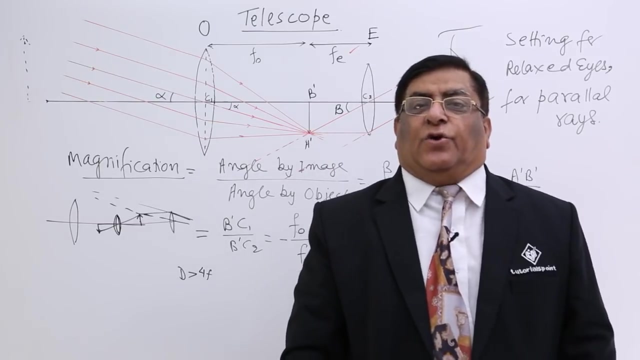 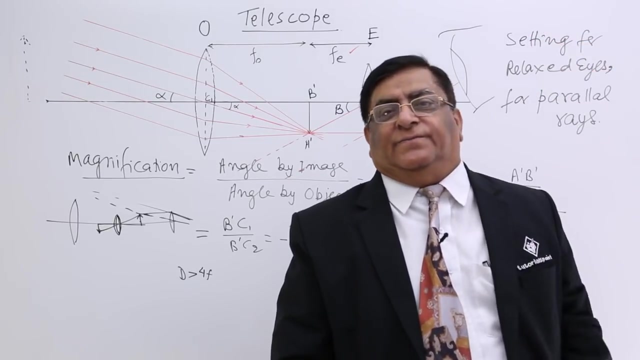 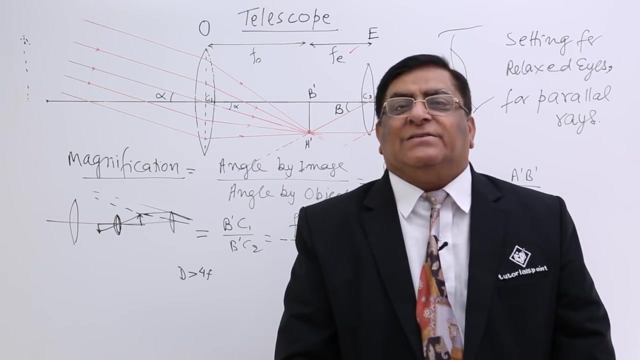 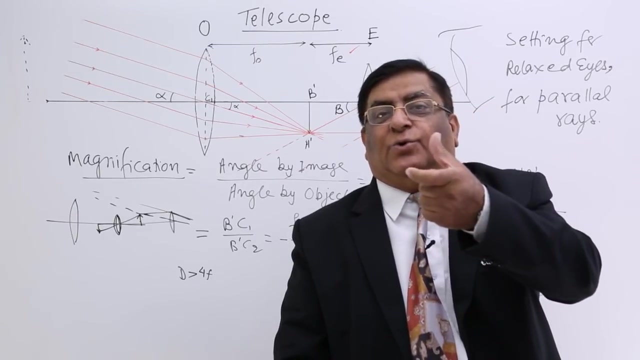 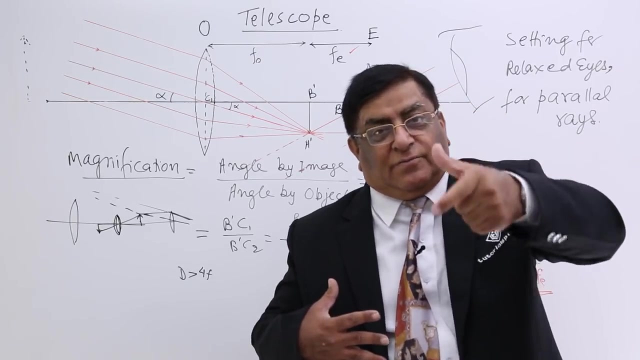 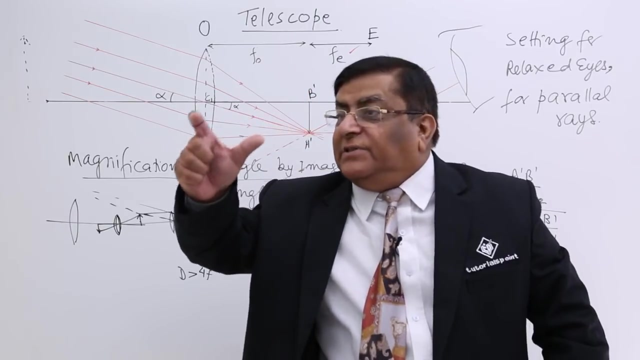 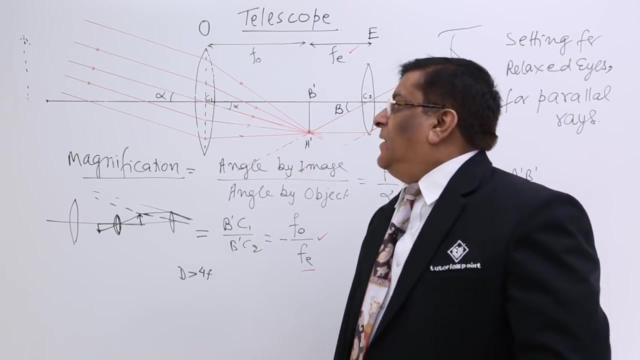 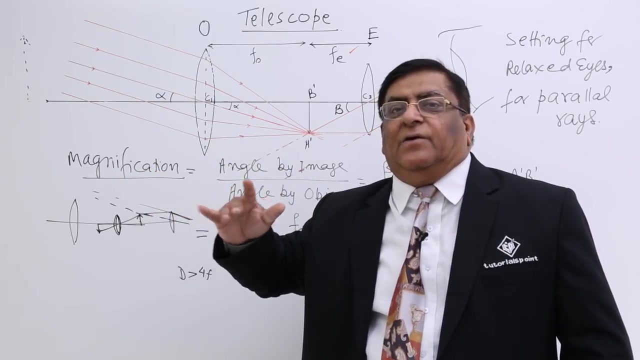 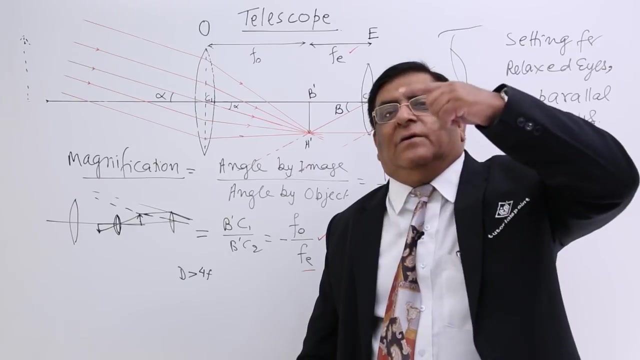 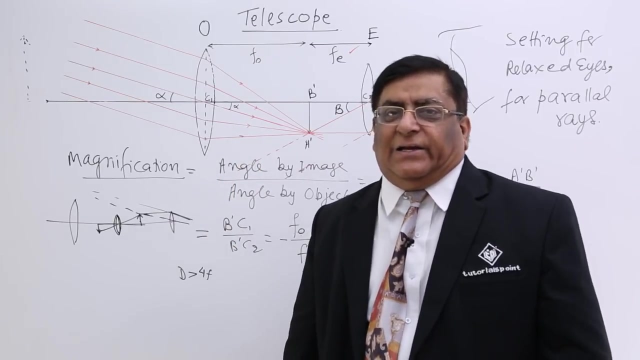 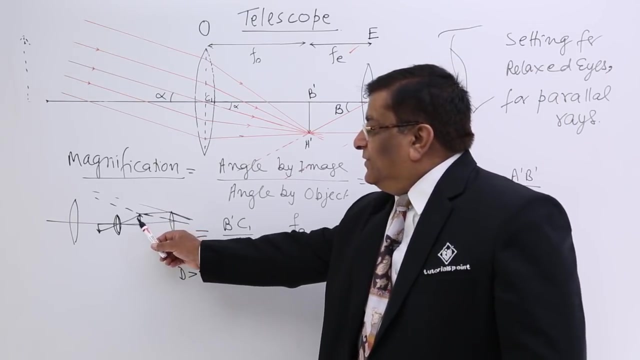 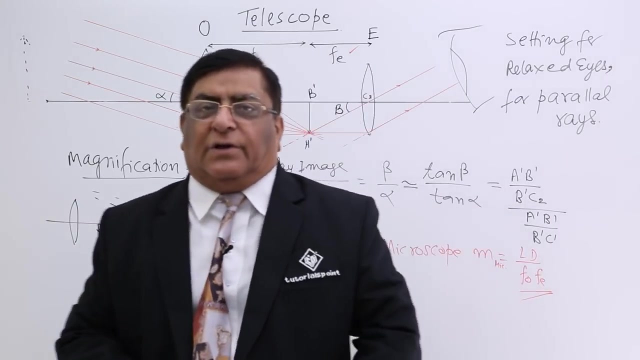 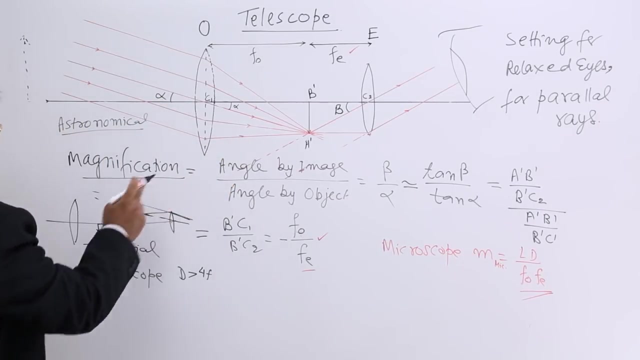 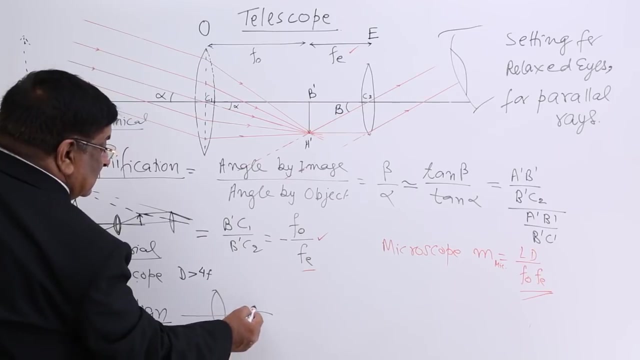 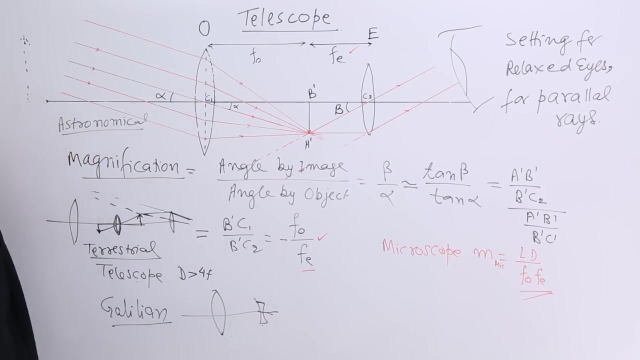 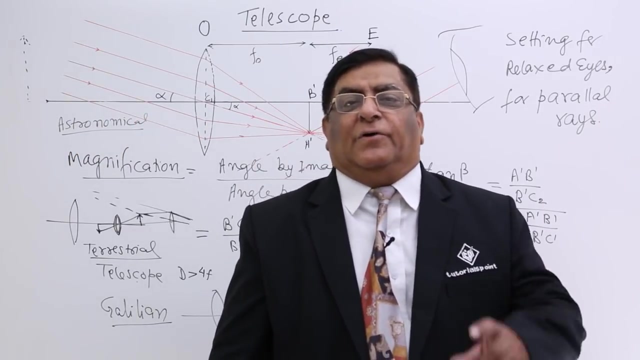 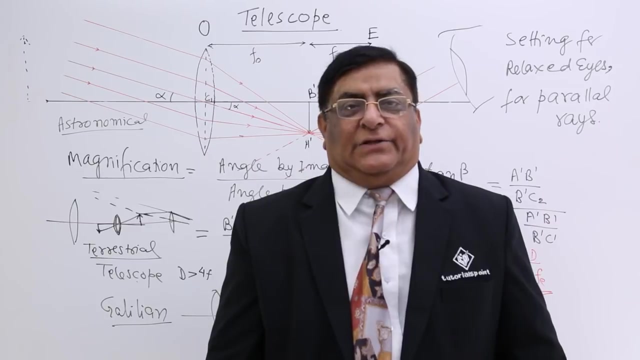 how we can rectify that.